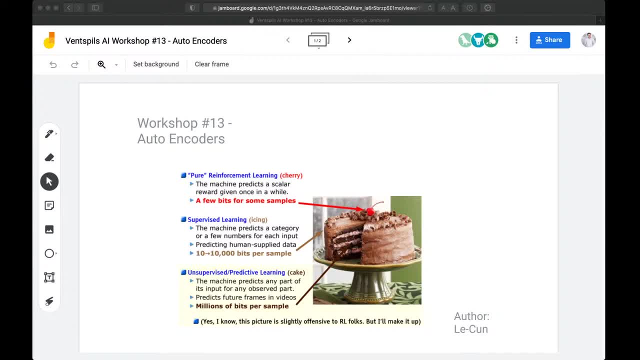 Thanks. Transcription by緞. Transcription by vitiligo. Transcription by vitiligo. Transcription by vitiligo. So from from the people who are here, at least at least two of you already have Okay batch normalization. So it's not really batch normalization is not around the zero to one, but around the standard deviation. It's. you could imagine it something like minus one one, But okay, so would imagine it's kind of a 20,000,000, the delay 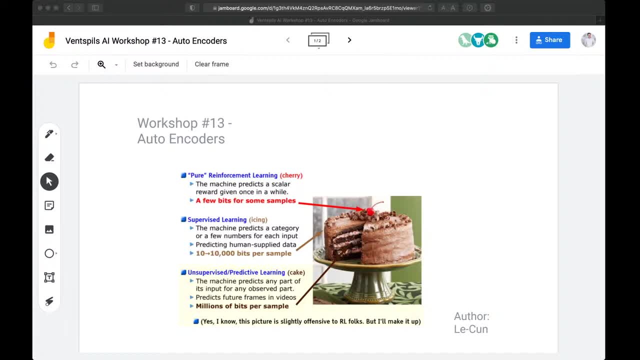 But overall it could be something like. But overall it could be something like between, say, 10 or 15 days longer, you know, just to filho put off, sometimes there is a defeat, something like minus 1 to 1. but okay, I will briefly touch the batch. 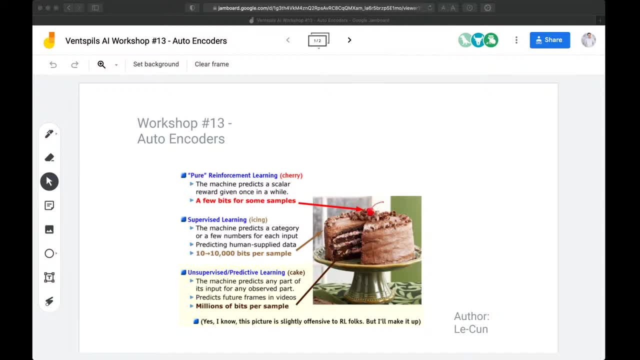 normalization and normalization techniques at the end of our today's session, because the homework will be kind of, I will give you the state of the art type of the architecture for autoencoders, so it will not be like totally state-of-the-art, but yeah, okay, we have used the not understood, so yeah. 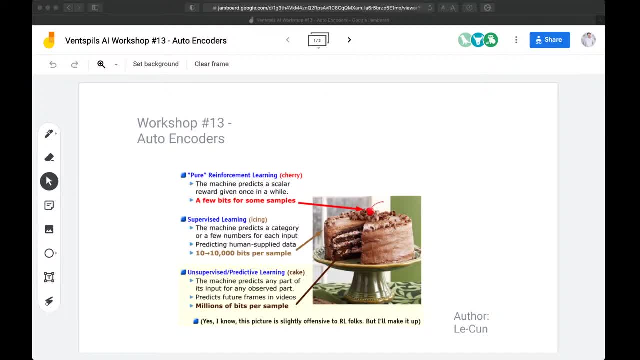 it is, as you understand, the normalization. so you want to place the features around the zero, so, and the batch normalization is kind of tries to estimate the feature space along the whole data set based on the batches. so it's not optimal. that's why, as I say, I will touch that in the way like that at. 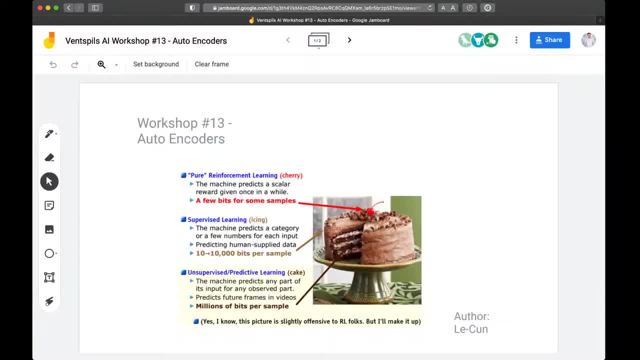 the end of this session. so the first slide this is: this is a. this is regarding the autoencoders. autoencoders do not require labels, so the autoencoders work without labels. you don't need to know what are the labels. you know, like we have supervised learning the middle part, the icing of 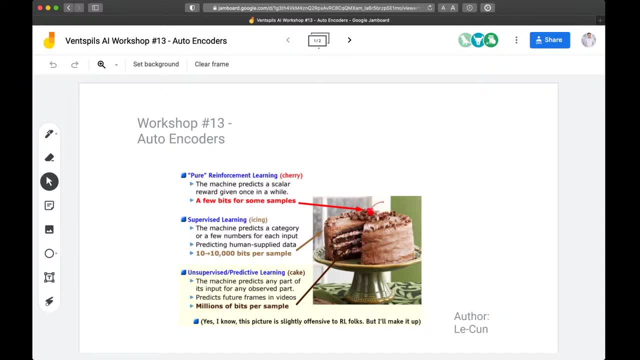 the cake. so this illustration is made by Lacoon, who is the one of the most important researchers in deep learning, so he was the one who invented the LSTMs. he was really influential also. so I'm not sure about LSTMs, but but the convolutional 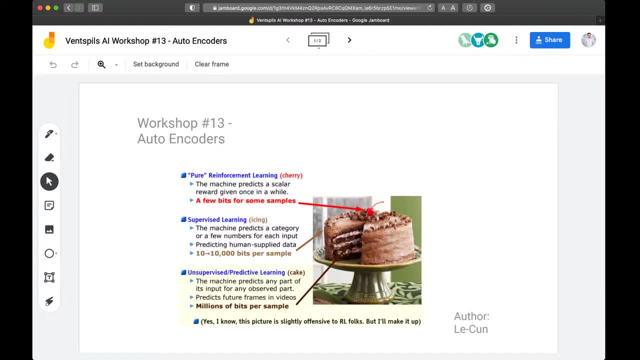 was was was his part. he also worked a lot of with energy models, a lot of them with the embedding models. so so he he gave this illustration that the icing- like in a cake icing, the chocolate part, that is supervised learning where you have the labels, then the reinforcement learning that I'm not sure like so 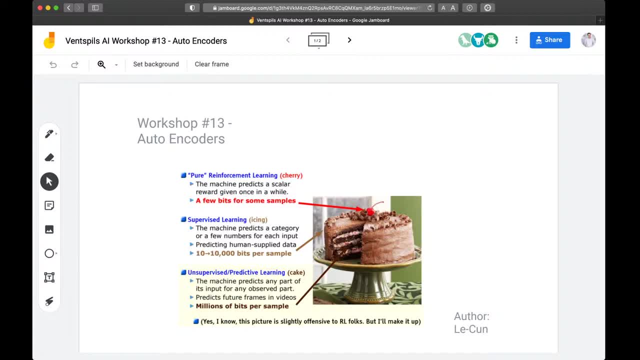 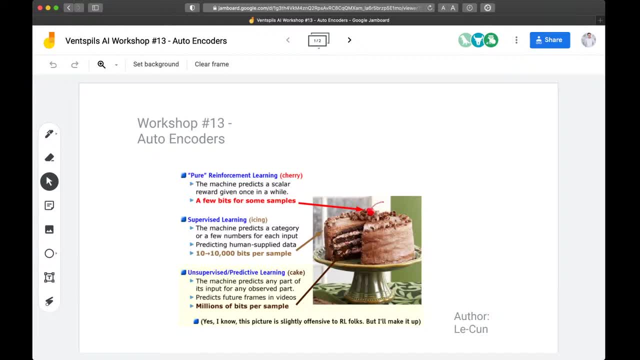 interesting to see how it works and I think it's very, really, really complicated and actually very small part of the deep learning- and then the huge part of the deep learning that is in the middle part of the cake, like the bread itself- is unsupervised learning. so that is like when the kid is looking at the events in the world and the children is. 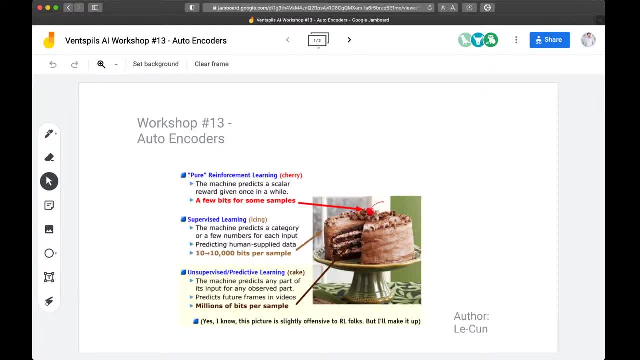 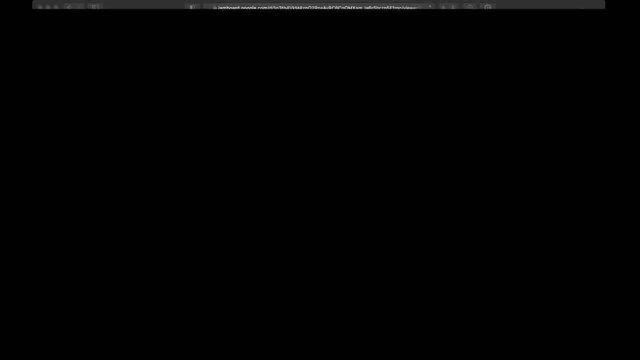 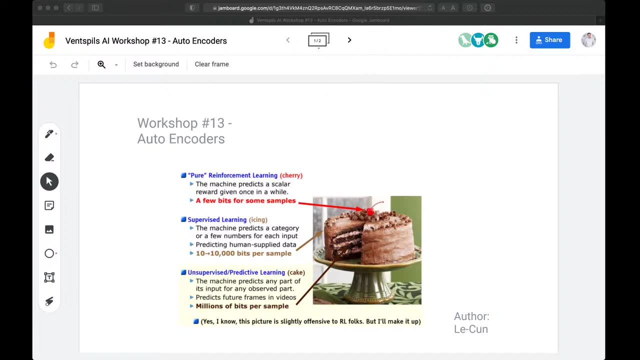 learning from them automatically, without any labeling. so this is, this is one kind of model that we will touch today, so let me introduce to the autoencoder. so i will make the next slide as well, and if you have questions regarding this part, then also please type in the chat. 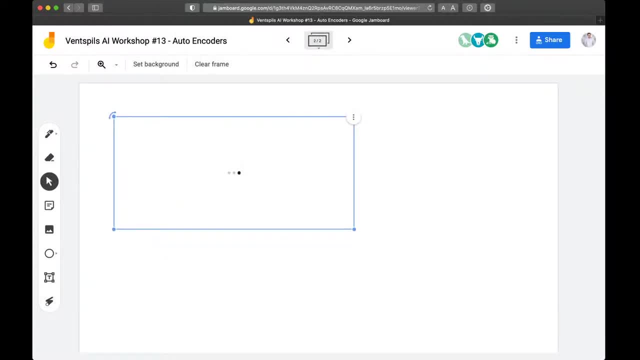 so the autoencoders, in a very primitive manner, looks like something like this: so they are the encoders. so encoders, we already know how to make. we already know how to make dense nets, resnets, all sorts of things. so we already know how to make dense nets, resnets. 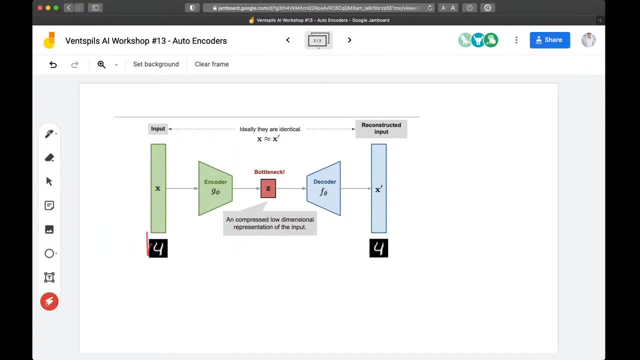 of stuff. so so far we have done this part till the bottleneck Z vector, latent space vector. so that is the idea that we can encode high dimensional image into low dimensional, 10 dimensional probability distribution that we can classify. but we could also compress this high dimensional image to 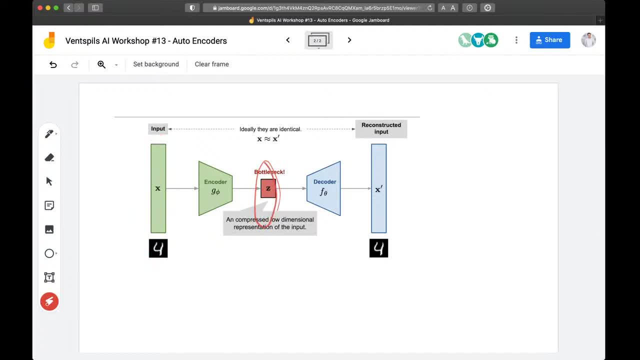 something like 32 dimensional latent vector, for example, or three dimensional or whatever, and then we can deconstruct the whole image just using the small representation and create something like this: so the decoder part, the color part, is based on transposed convolutions or there are more modern approaches at the 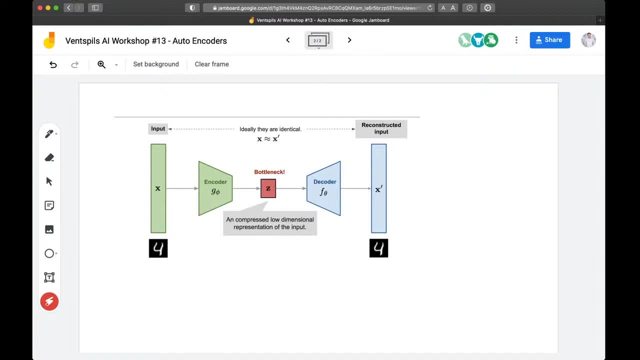 end, like in the homework, I will give you modern approach, how to do this by Nvidia, but like nobody actually used in modern models: transpose the convolutions they have, checking the convolutions and then the decoder part is based on patterns and all sorts of problems. So the idea is that you have input X here and 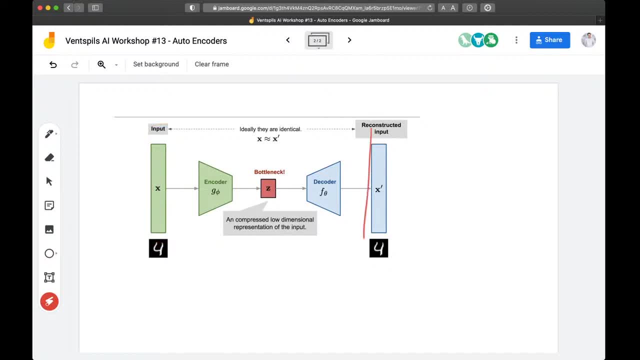 the reconstruction is basically the same X and you try to learn this Z vector so that it encodes everything that's important about the X in very small vector. Hopefully it's clear. if it's not clear, then please type in the chat exactly what is not clear. but yeah, so that's the main. 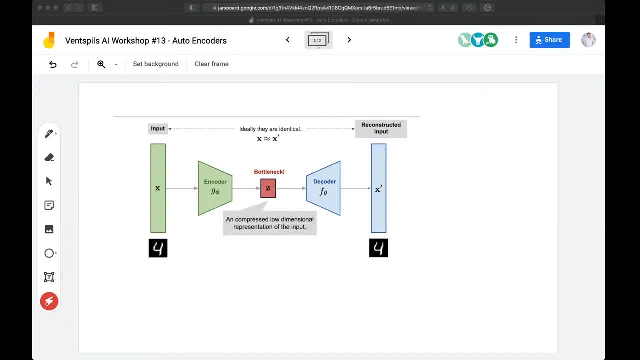 idea and maybe the other illustration. if you have better illustrations you can also share with me- but is something like this, So let me see. so you probably know that there are dimension reduction techniques, so these are like algorithms, methods for reducing the dimensionality of the vectors. so one of the method that is not 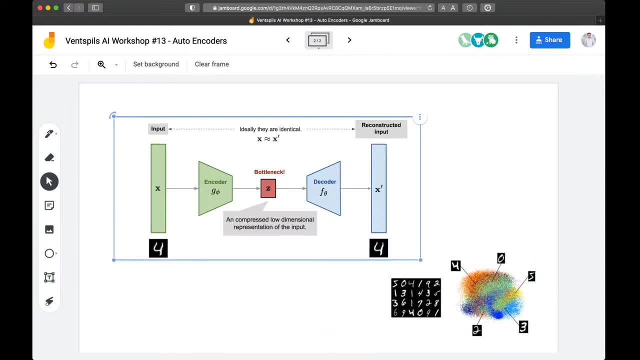 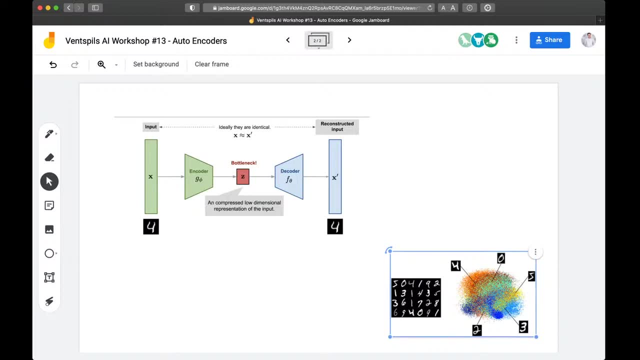 good is the projection method that we know by doing the dot product. remember that by doing the dot product we can like have the input of 32 dimensions and output of just three dimensions or two dimensions or what we decide. but there are better methods. for example, principal component analysis, that is, selecting. 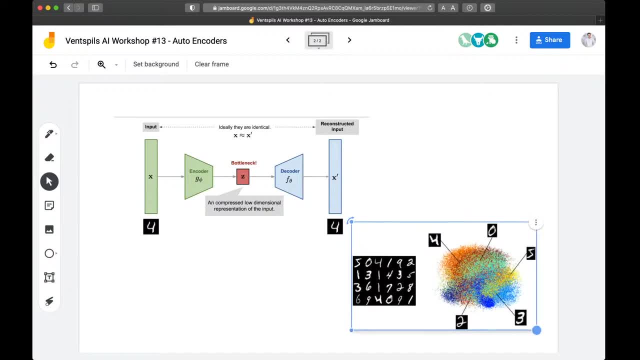 the dimensions that holds the most variance and then projecting that on that dimension. this is like using PCA, but there are also T, SNA and the one was UMAP or something. so there there are quite a few methods, but the idea is is following. so if they have perfect, 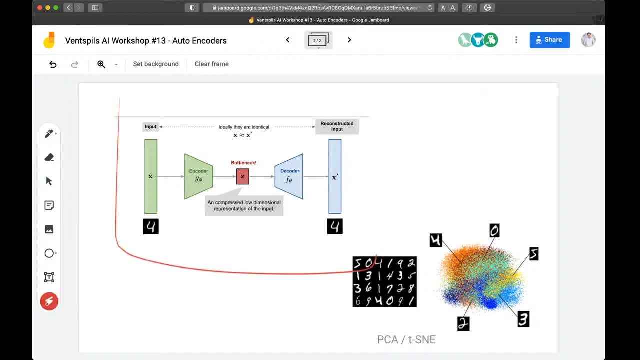 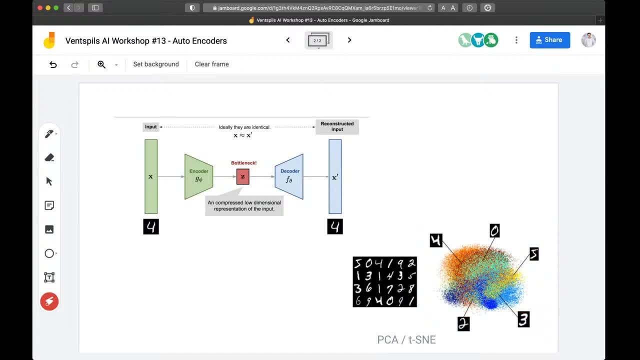 three-dimensional space. all of the samples that are force, like this sample, this sample and this sample- they all cluster together in one cluster and we have not told the model that they should cluster in this place. but the model optimizes all of this latent space in the manner that it generally like, tries to place items in a 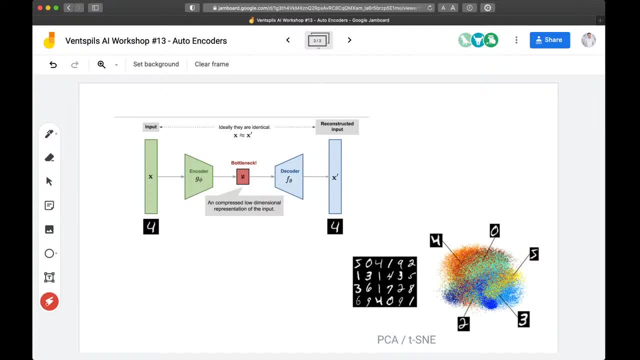 cluster. so that would be the least resistance for the model to calculate back the decoder part. and there are some methods to encourage these clusters to be aligned by their similarity. but this method is not encouraging that but at the same time it still gives you the clusters and the approximate. 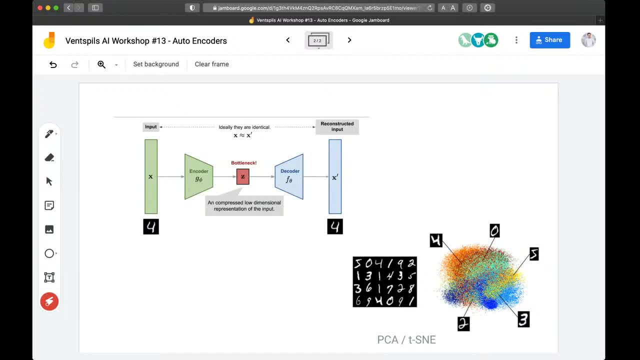 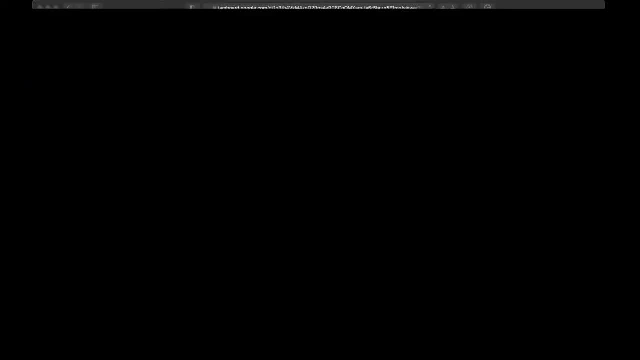 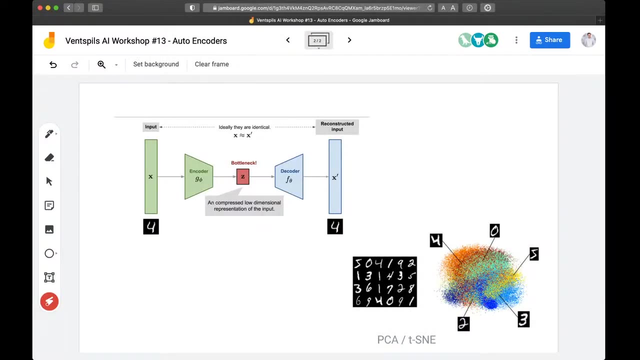 locations of same class images. basically you- and this is quite significant, because we never told the model what are those classes- the model learned these classes by itself. so is it clear so far? what is the autoencoder and what is the advantage of the autoencoder? so, if, if, 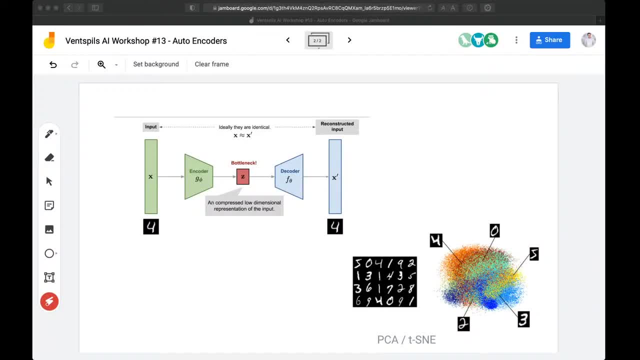 what I said so far is clear, then type in plus, if not minus. is it clear so far? plus, minus? then I will follow up with some few things and then we'll start coding this stuff. by the way, all of this information is we also included in the preparation? 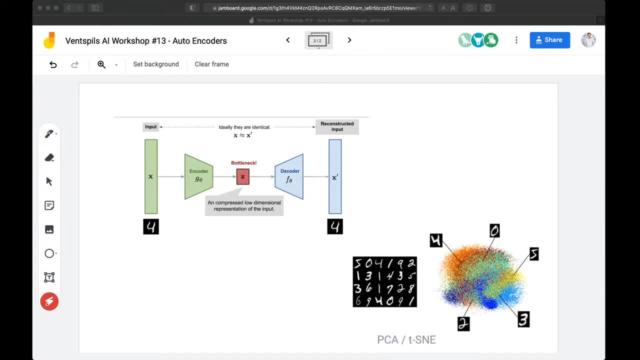 materials for those of you who read it. so I have two pluses. we have seven people online. I need more pluses to continue, or maybe you can have question. so if it's not clear, then type in the question, so maybe I will also add explanations, some explanations here. so this is the middle. 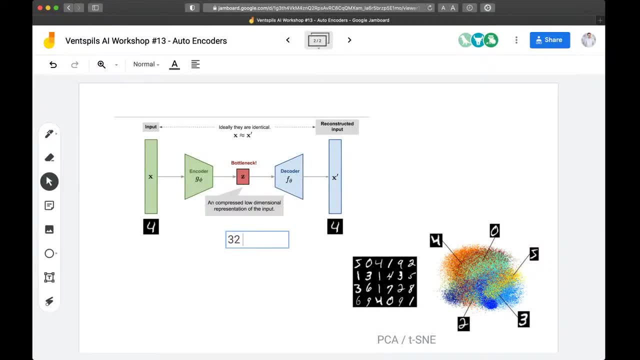 it could be 32 dimensional Z and then we display this using. so this is a three-dimensional DIMM reduction, just for the visualization purposes. No, AutoEncoder is not the really principal component analysis, because AutoEncoder, so the PCA, is the method for displaying these embeddings into. 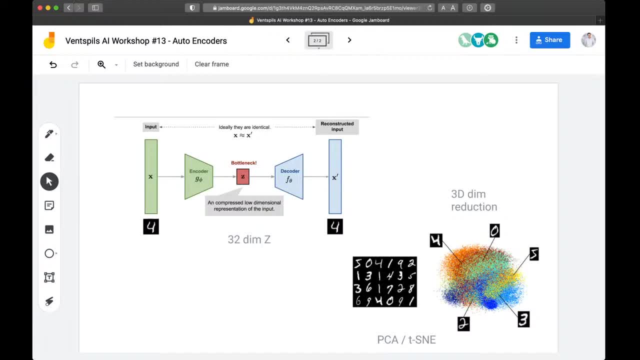 visual representation that is understandable by human being. otherwise, if I give you 32 dimensional Z-vector, it will be not possible to visualize it so that you can understand it. So that's why we use PCA or TSA or some other this techniques for dimension reduction. 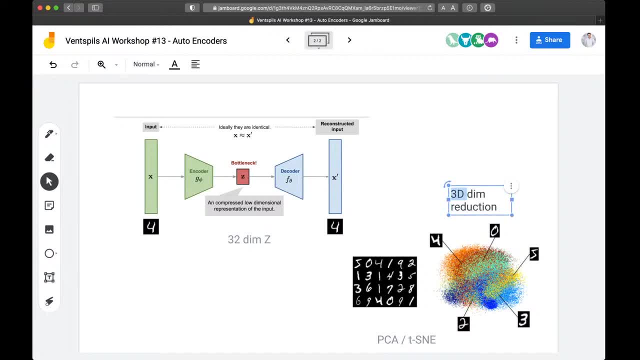 three dimensions and only then we can display that. so I'm trying to just give this example, so that you have 32 dimensions coming in right and then you get, with a dimension reduction algorithm, something that's in 3d, just for visualization. this is not part of the model, so I'm just want to emphasize that. 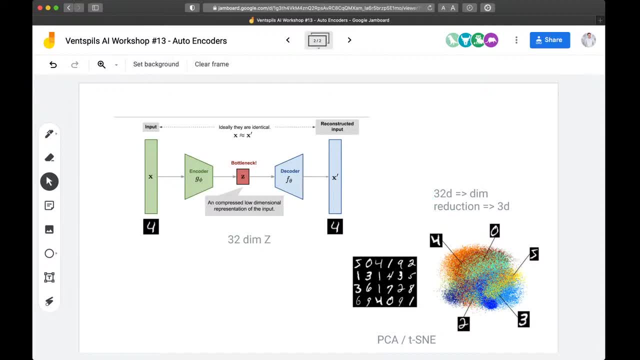 we are working with high dimensional Z vectors. if you want to visualize them, we reduce the dimensions. but if you want to use them for, let's say, re-identification of samples or using the embedding vectors just to find out which sample is the closest one, we would not do the PCA. How, for example, would you get? 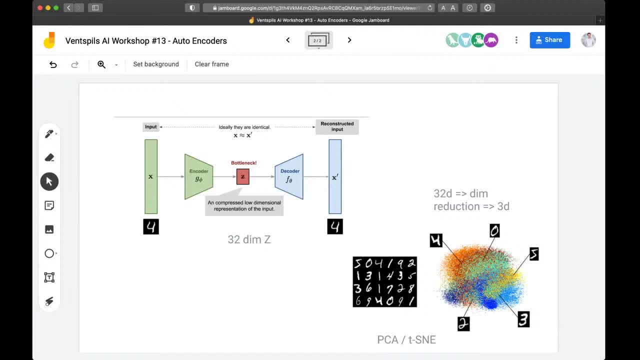 that picture out of the model. You would not get that picture out of the model. you would get the list of 32 dimensional vectors. then you would fit this to the PCA, find the principal components and then project on those components, those vectors, to see this nice 3d picture. that is why I'm trying. 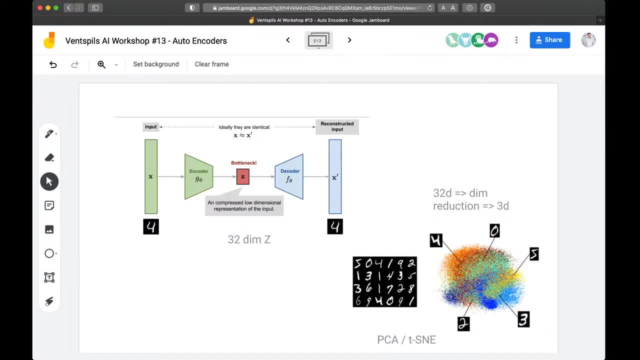 to explain this part, because I think without explaining this part maybe you don't understand why at all you need autoencoders. So the one thing that's missing here from the explanation is that let's say: this is our like. let's say some training data set or inference data set, and now, if we get some example, 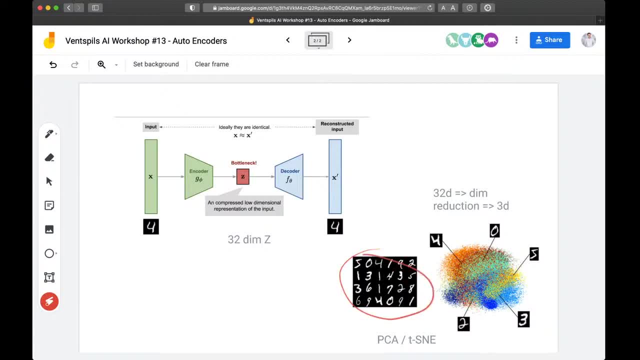 that was not inside here. for example, some person just draws manually letter four, right, the person draws letter four and you have this image. then you encode this to the Z vector- just this part, not the other part- and then you would place that somewhere in this dimension like the high dimensional space, and 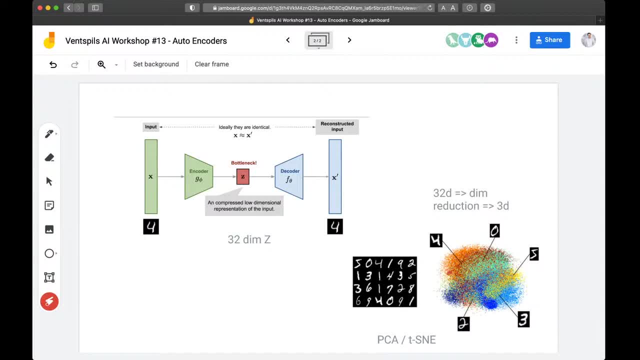 what you expect, that this point in this high dimensional space will be very close to the cluster of force, and that way, basically, you just created classifier without any labels. so basically the other way, how you can use this, is for, let's say, face identification or Apple face ID or 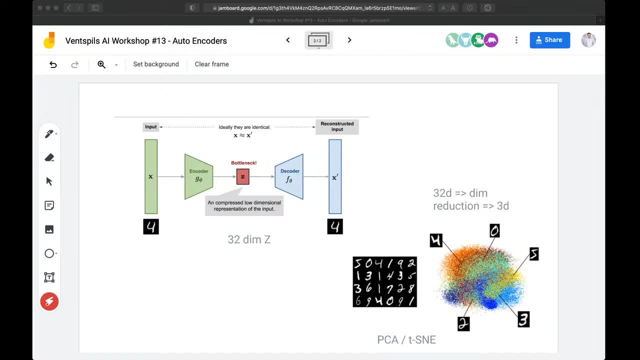 something like that. so let me find some picture face re-identification identification clusters. so there are quite a. so this method would be very weak face re-identification method because there are not nothing that enforce the arrangement of the clusters in the in the high dimensional latent space. but if there would be some 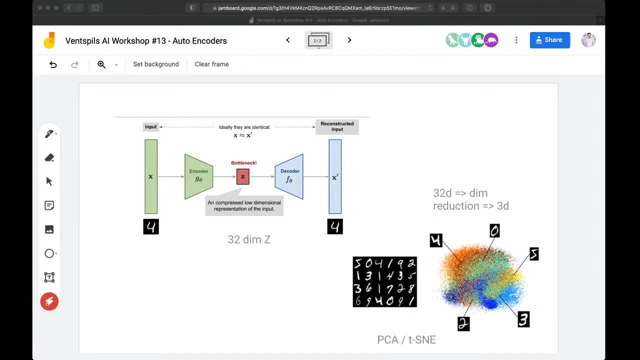 enforcement, it will work better. but still like, basically, if that, if this is not a scenario of one-shot learning, it would still give you quite nice clusters. so just me, let me find it. PCA. so let me see can I find some example. okay, I cannot quickly find nice. 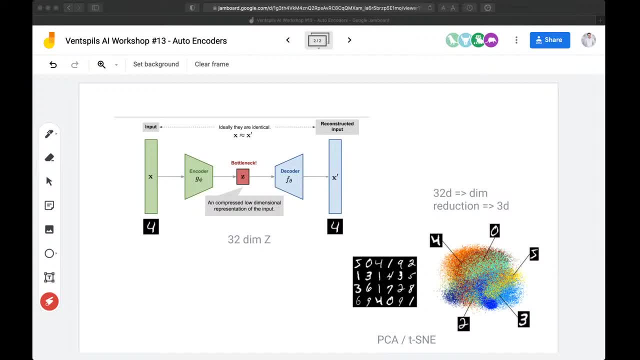 picture of the clustering faces. but basically you can imagine that if you, if you have trained your model with some faces and then you give some new face image, then you can check where it stands in this cluster. the other nice thing that interesting, that I'm not sure like if you get it or not, is that you 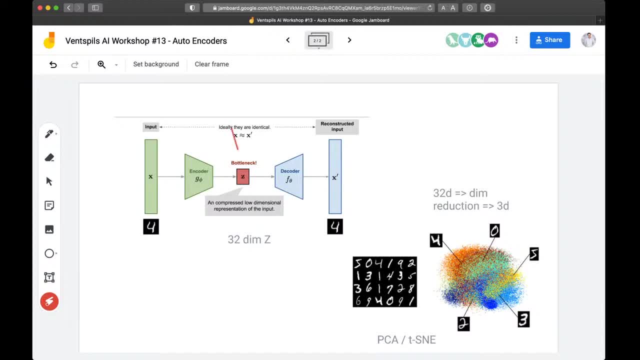 can also create. this will be your first generative model. basically, you know GANs and stuff like that. so if you sample Z vector, so forget this part. if we train the model and then we delete this part and then we just take the some kind of average vector of force and then add some. 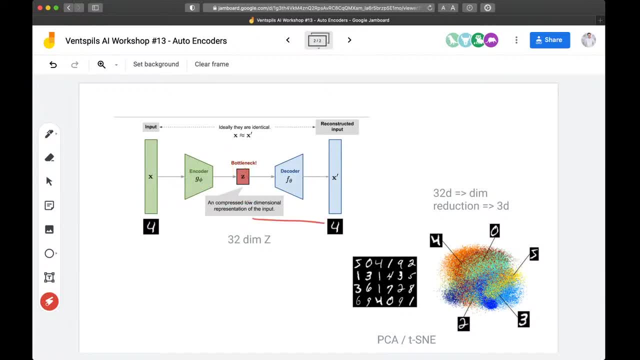 noise. we can sample new force, like in different styles, just by using the only this part. so this is quite powerful. you already have the capabilities of either re-identification and also a generation. so this is, this is quite cool. okay, so we'll move to the classroom in the classroom and we'll open now the 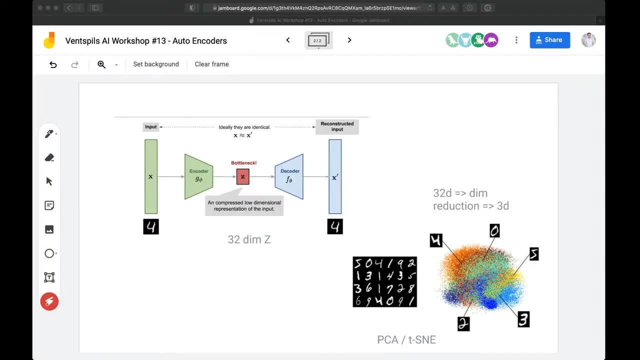 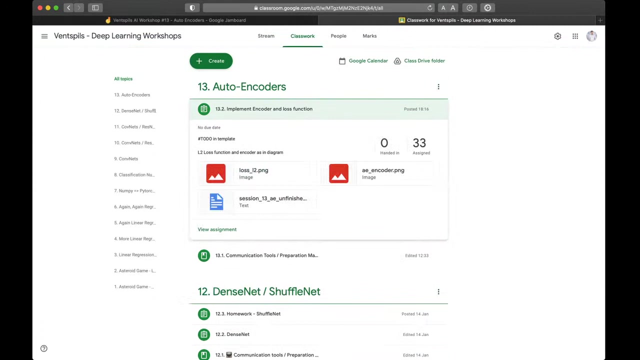 task 13.2 with with the two to two tasks that you need to do there, and you should be able already to complete those tasks because they are quite easy. so let me share you this screen, so if I open this one, so there is a classroom, task 13.2, and you need to download the template and 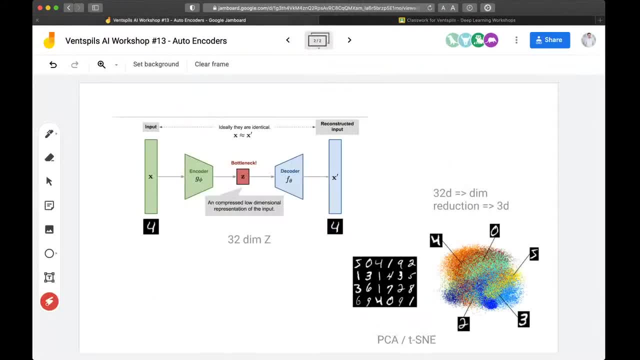 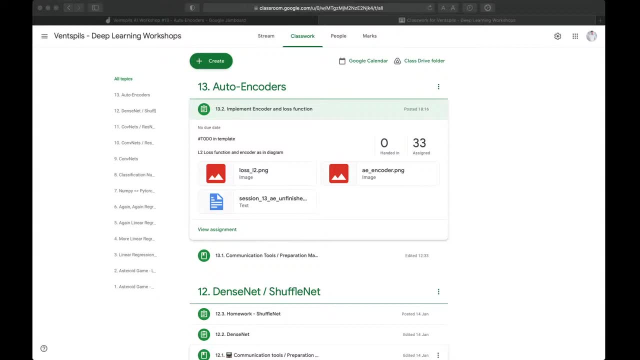 you need to. first, what you need to do is to run the template, because otherwise it will be very long before we can start working with it. because, because we- I'm chosen the data set extended MNIST. that is, like MNIST with, but with more images, with more letters and numbers and all sorts of written signs. so if you 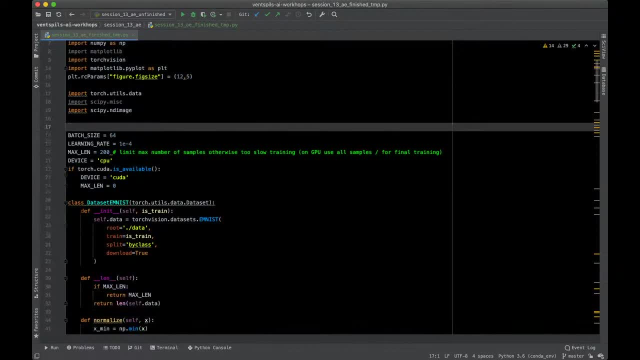 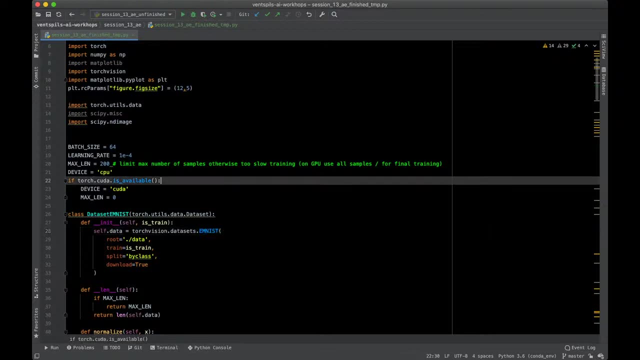 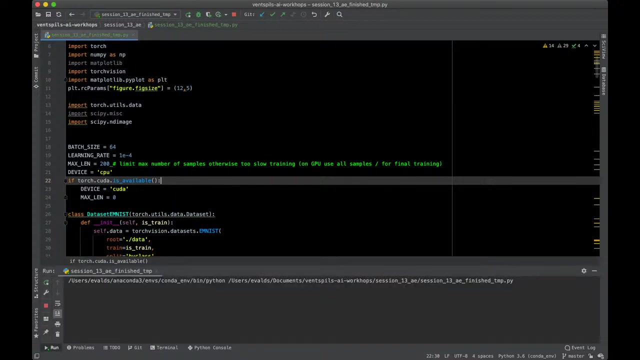 download that template. and then here I have this template. see, there is a data set extended MNIST. so if I run this one with, just with the run, I will see that it is downloading the the images. so please run the this code and so that you download this dataset. I stopped it because I already downloaded. 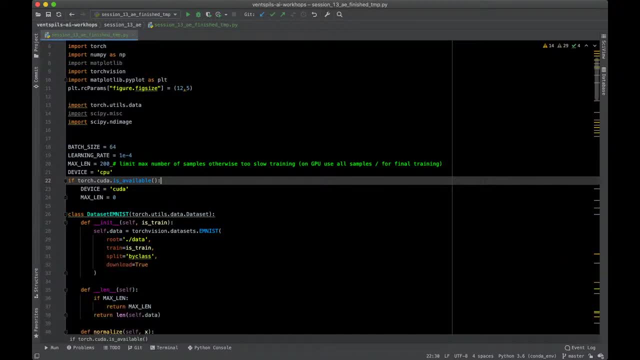 so my question will be two parts. so first let's start with: do you have a template ready to work? 13.2. so this is my first question. type in: plus, minus or some question. and if you, if you type in plus, immediately press run so it starts downloading the this data set, because it might not be too. 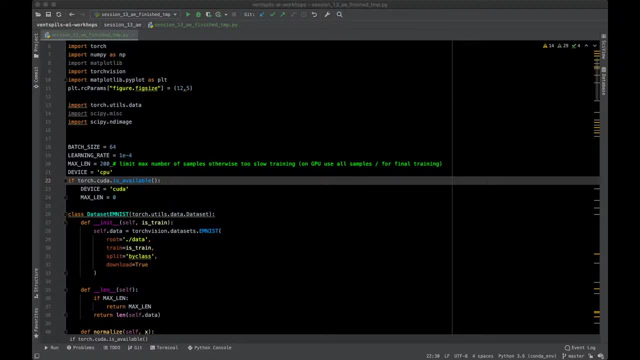 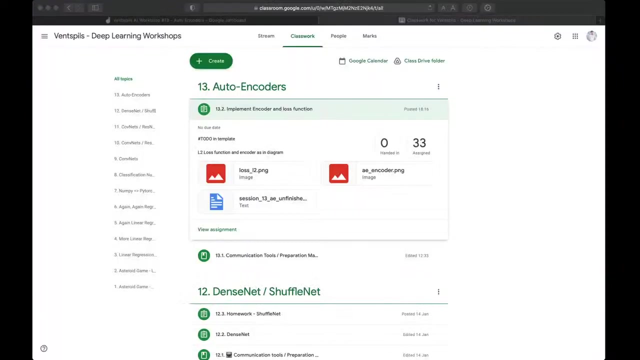 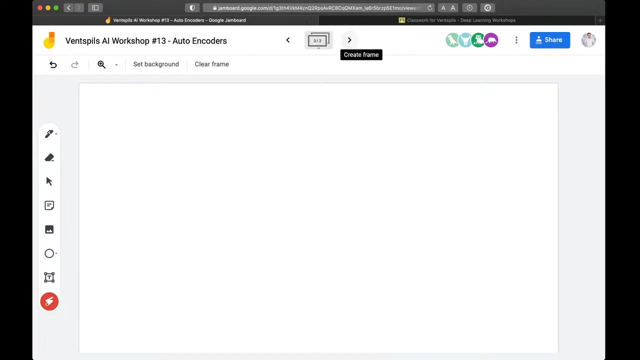 fast, so maybe you will need to wait five minutes or so. so please do that and let me know if your template is ready for work. meanwhile, I will share some stuff on the Jamboard, so basically, where I gonna share here is just just the same things that is requested to do, so while 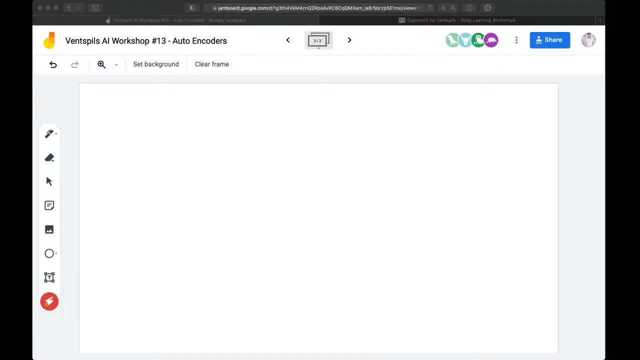 you are downloading the this stuff that you have on on the task, like, like, I mean the dataset. while you are downloading the dataset, you can already start implementing the tasks. so one task is really simple. so one task that you need to do is to implement the loss function. so the loss function for this case. 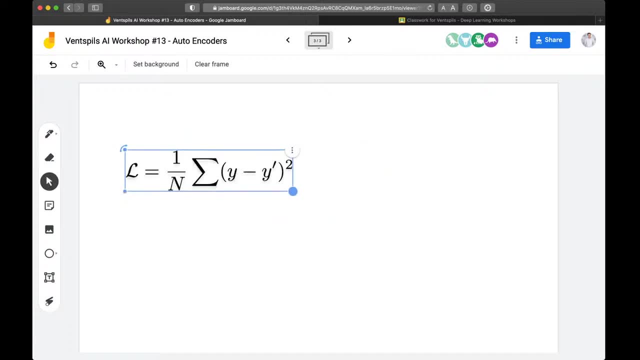 we will use the mean squared error. so you implement the loss function and you also implement the model, the encoder part. so when you will run it, you will see funny pictures in the decoder part. that is what it is expected. so the funny pictures of the encoder part are expected because 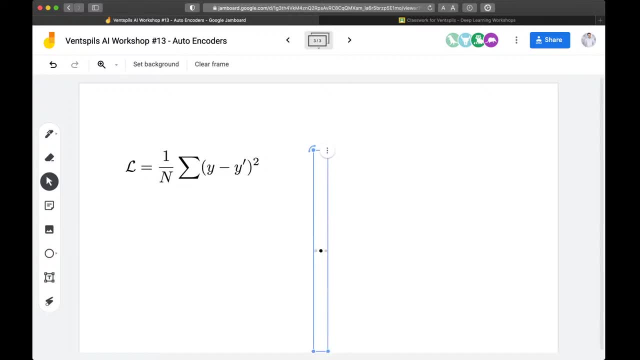 we have not yet implemented proper decoder. so let's see. so this is the module that we need to implement. it will be much easier to see if you look at, if you look at the like, if you zoom it in. so this is gonna be the task. task thirteen, point two. so you have the loss and the. 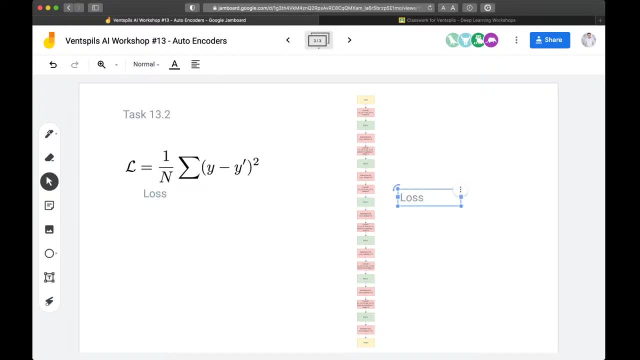 encoder- I will try to improve this image right now- and what else we can do. so, yeah, you should start coding that and the submit when you have done it ready, because otherwise it will be too slow with this, this tutorial workshop. so my next question will be: so have you missed? downloaded yet and again plus. 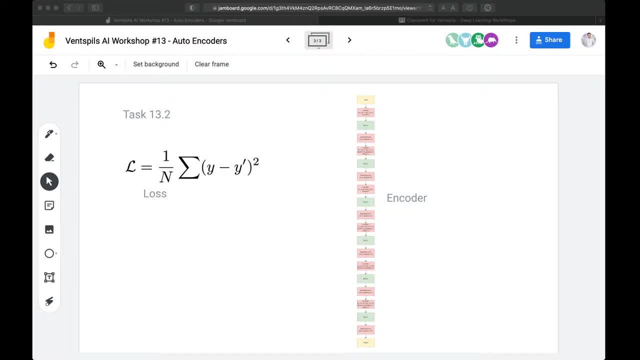 minus. so from from previous question, I got five pluses. so that's good. almost everybody is ready to work. and then the next question is the: is the downloaded already? well, well, I'm waiting for that question, and while I'm waiting for your code, the image is very low res, yet us you. you think you say that in the task it is. 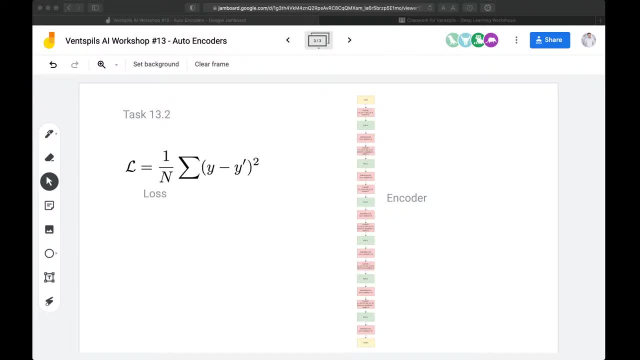 of low res. let me check. let me check so I see that it is not low res if you download it. but but let me see. so if I, if I press save as this, image you what like that. but there was some airbottom to download it somewhere then 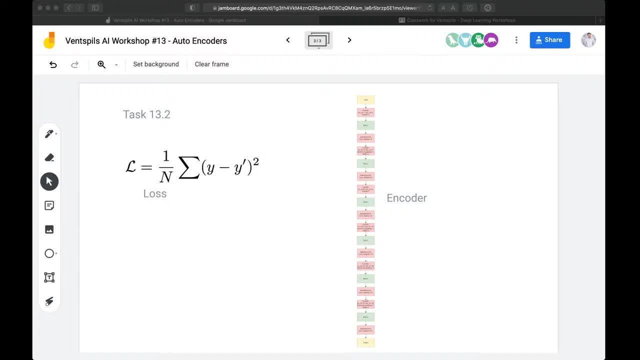 it is a proper size, but I will also improve it, so I will maybe split it in a month. yeah, yeah, I'm jan board. that is lower their own law res because the John board is small. so i will try to fix it quickly. but sum, meanwhile you can start working. 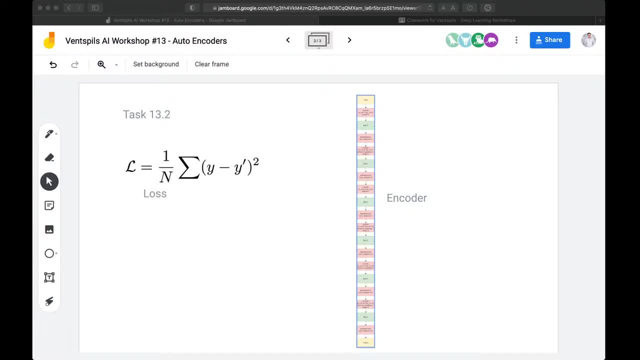 working with the image from the Google classroom, so you should not have serious problems implementing this model. so I will wait for some of you to finish it already. So, as I said, don't worry about the output part, so the decoder part. now it's not finished. 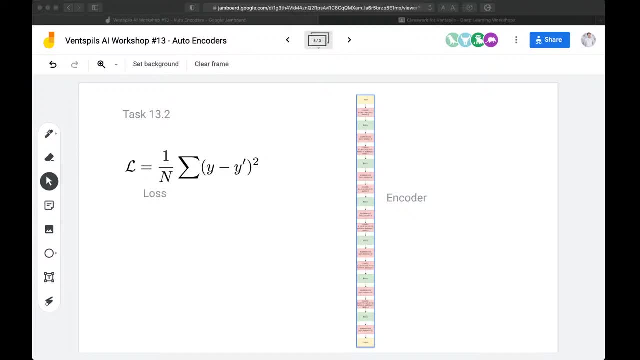 yet it might look funny and not really beautiful, but that's, that's no problem. so okay, I cannot yet fix it like that. let me think I will find a way how to improve the image quality here. okay, I will split it in two parts most likely. so if it's something not clear what to do, then also please ask. meanwhile I will prepare. 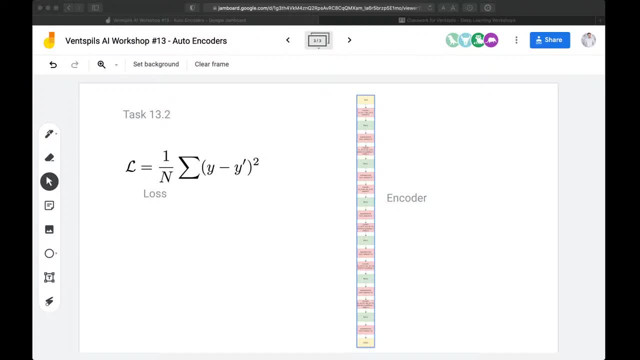 the small update for that image. you can go ahead and read it for yourself. okay, you can go ahead and read it for yourself. okay, so you can go ahead and read it for yourself. Thank you, So the update will be very soon, So in just a second I will update this one. 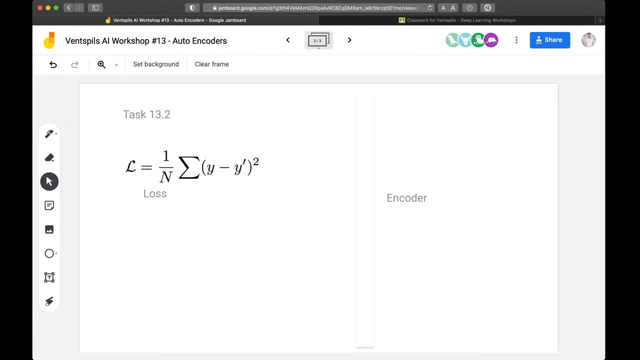 and then I will look at your questions. So I prepared a better version. Oh man, what is this? So it didn't work like that. Just a second: Okay, like that. Yeah, so the encoder. the encoder is looking like that. 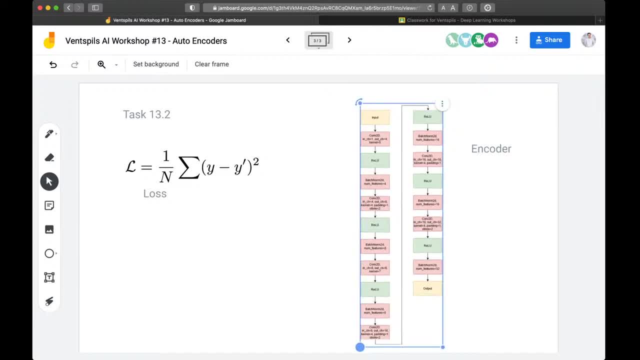 so I just split it in two parts so that it's visible a little bit. Okay, so we have autoencoder here. I see one minus with regards to. So I propose that you already- all of you- start coding those tasks and don't wait for download. 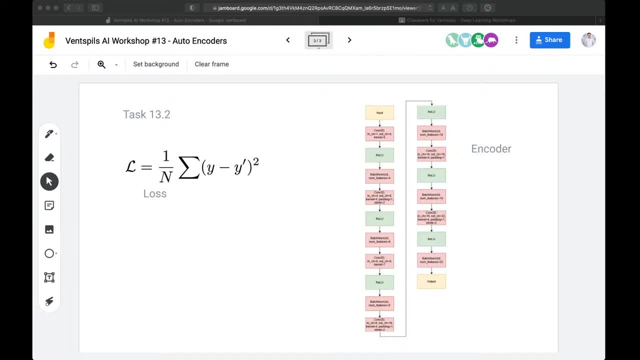 So when it's downloaded then you can run it and test if you don't have bugs. But meanwhile please start making those tasks And I will also in, like, let's say in five, ten minutes, let's say ten minutes. 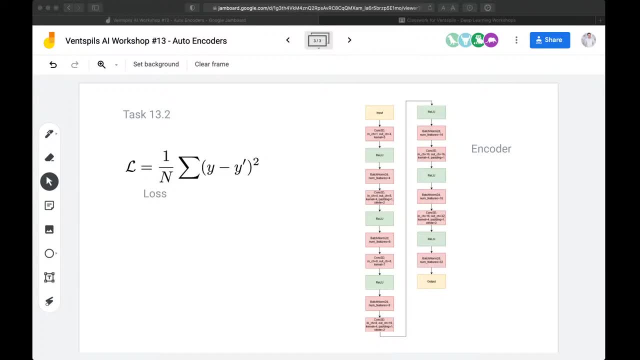 we'll start showing how to do this And hopefully some of you already will be able to submit this task. At this moment, nobody has yet submitted this task, So I will turn off the microphone, So please try to do this. 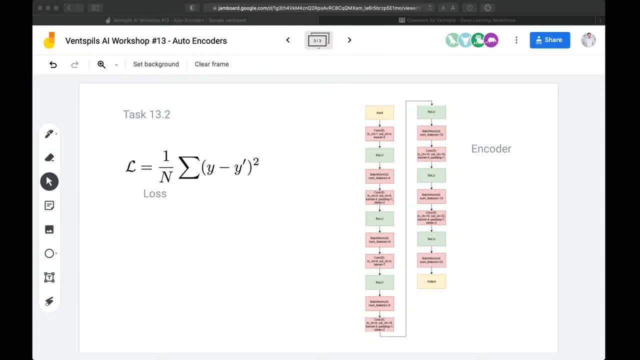 Even if you don't know how to do something and you try, then please submit what you are able to do, So then I understand what are your capabilities and I can help you out. Or if you have questions, then type in the chat. 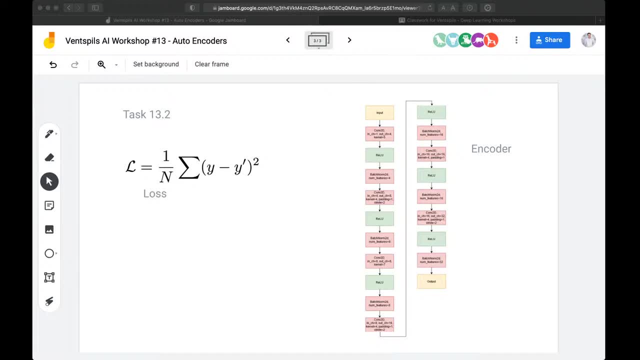 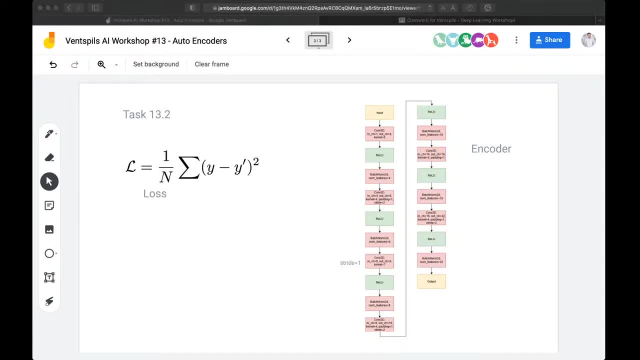 I think yeah, And let's see: Okay, Okay, Okay, Okay, Okay, Let's see if there is some other place where something is missing. So I think everywhere where you don't have stride written, it's a stride of 1.. 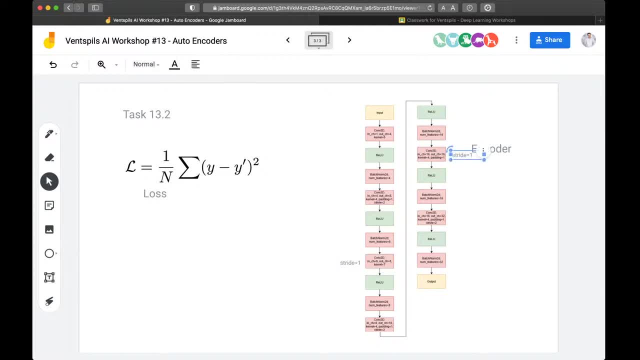 So stride of 1 for the first one, again stride of 1 and let's see, do we have any other place missing? so I think not. so just follow up. So in general, like you can even make a little deviances from this task, as long as your encoder 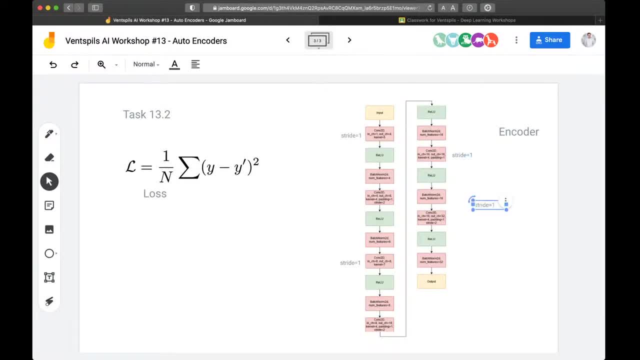 at the end produce the embedding of 32 dimensions. So here should be the output, should be like basically: so this is going to be, the output is going to be 32 by 1, by 1 in general, And if you flatten it then basically the output should be flat, would be flat embedding. 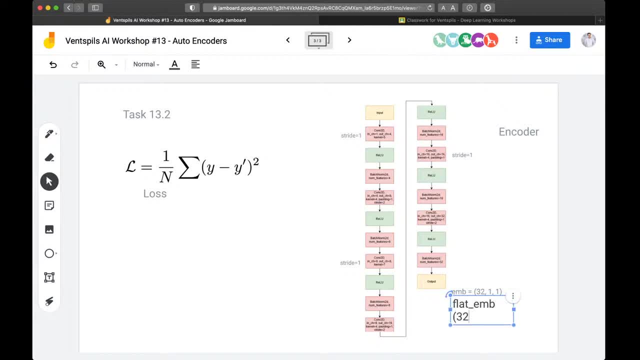 would be just 32.. So this is what we want. we want this embedding that we can use in that beautiful like space Actually, like I probably will do in the homework- the task, so that you can create this PCA space or some other dimension reduction method. so you can look at those embeddings. 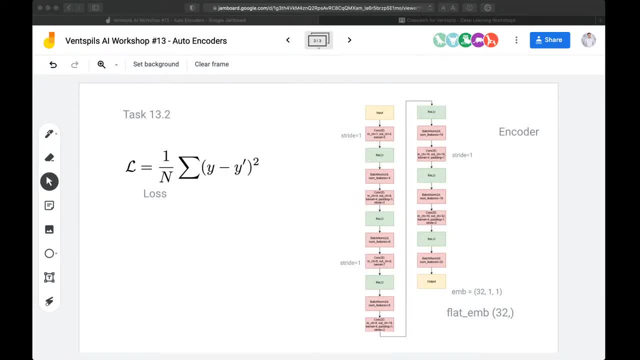 Right now nobody has yet submitted the task, so we will still wait a little bit. Also, let's do another round of a question, So let's try again. so have emnist already downloaded? So this is like the first question Plus minus: is it still downloading for you or you already got it? 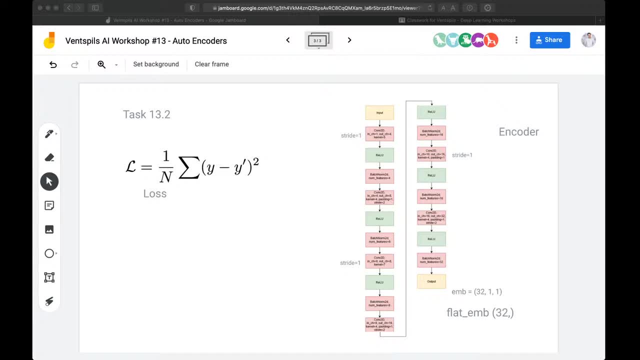 So if you got it, please type in plus. if we have done some problem, then please type in what is the problem. Okay, so let's see what we'll get. So let's see. So this is like the first question, Let's see. 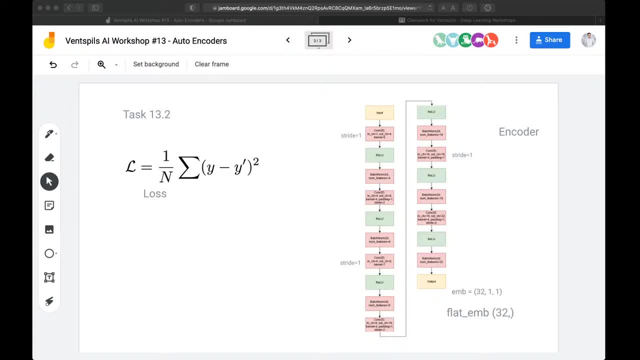 Let's see. Oh no, So this is like the last question. Is it still downloading? Yes, Okay, Thank you. Thank you. So I see some problems here. Let me see. Hopefully the problems will not be related. 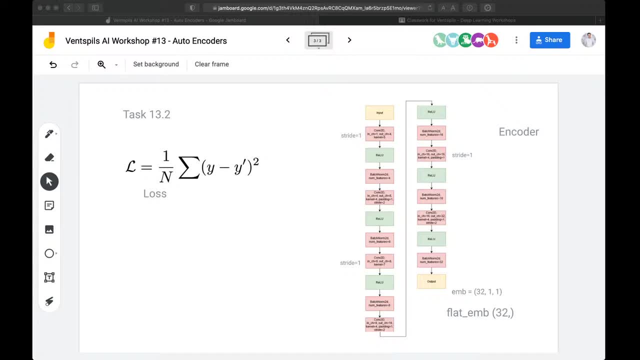 to the data set. So I have 80% for Kirill. The problem was that I have used mobile data right. There are some pluses. Then we have RL on loss value. Only element can be converted, So the 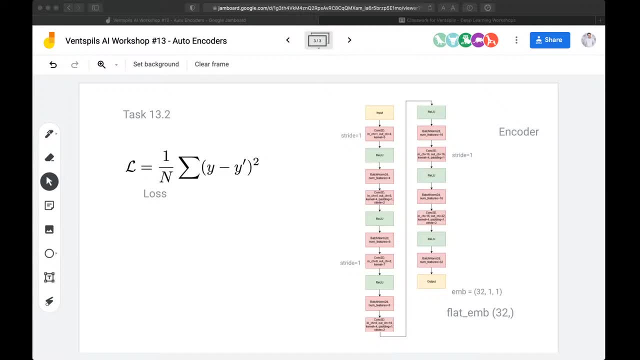 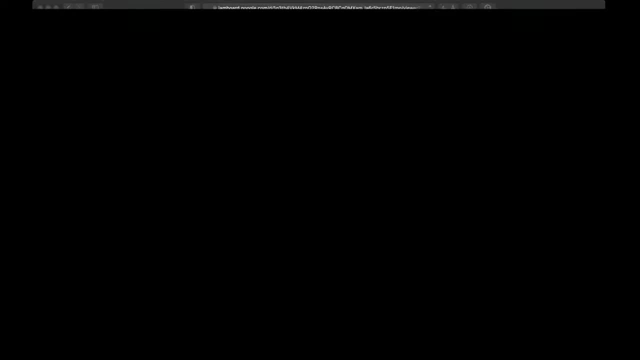 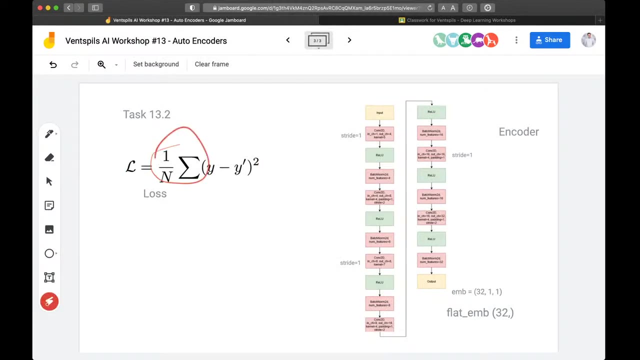 the Lee error means that he did not implement correctly the function. So the function is: if you look at the function, it means there is a summation, summation and then division by the number. So basically this is a mean. 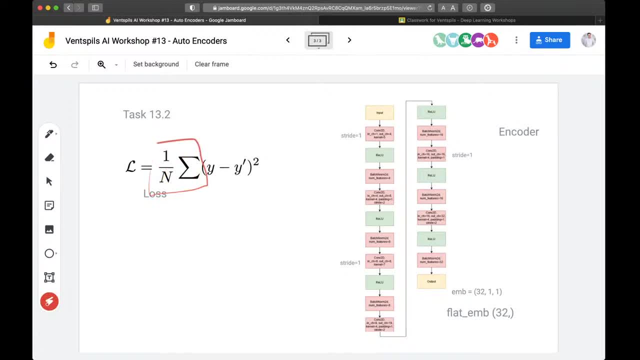 This is mean. So if you, if you calculate average mean value of these vectors here then, or the matrices, then you would have just one value and then it would work. So if you don't have just one value, that means that this equation 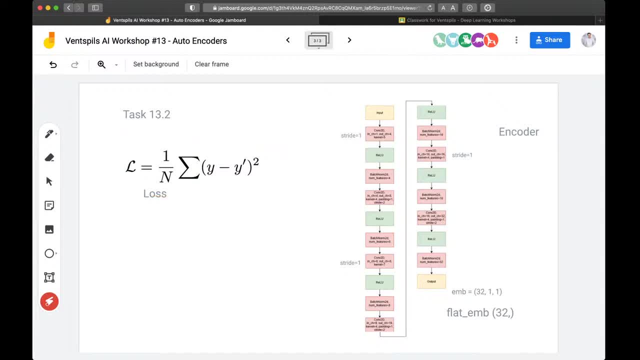 is not implemented correctly. So please look carefully at the equation, fix it and then submit it, or submit it what you have or like, if you can, if you don't know how to fix it at all, So you can submit what you have, then 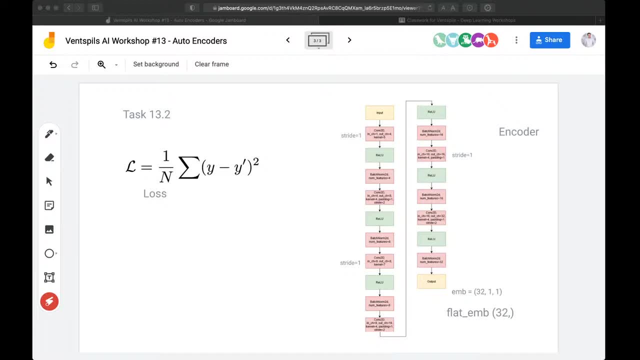 So let's look what is here. So what do we have? So the Christophers is already submitted The task, so that's great, We're waiting. I see that some of other guys are also quite soon ready to submit something. 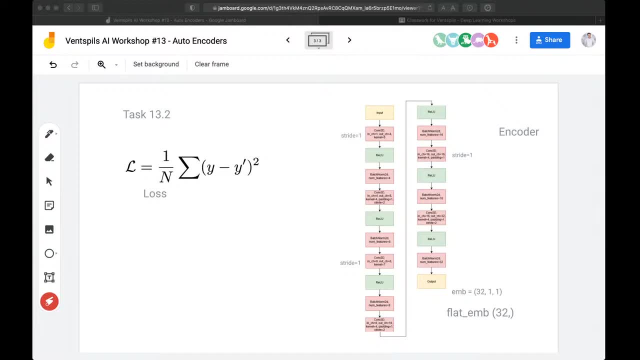 One thing that you will notice that the visuals that we have displaying after the every epoch. they are not perfect because the class names- as I found out that for extended list- are a little bit mixed up. We'll need to find the correct class names later. 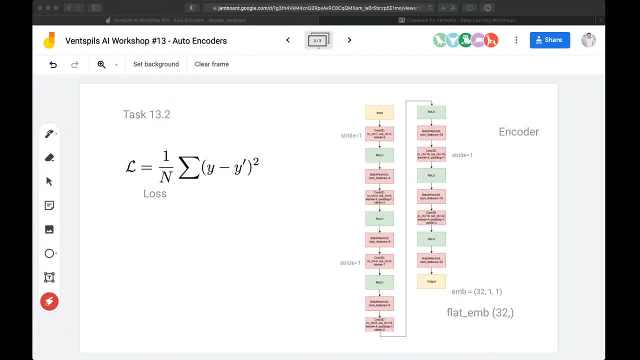 So I will check what the Christophers submitted Seems great. I like it. I think in general like what: if there is no error of what he submitted, then it's basically great. So okay, I see if there is yeah of. 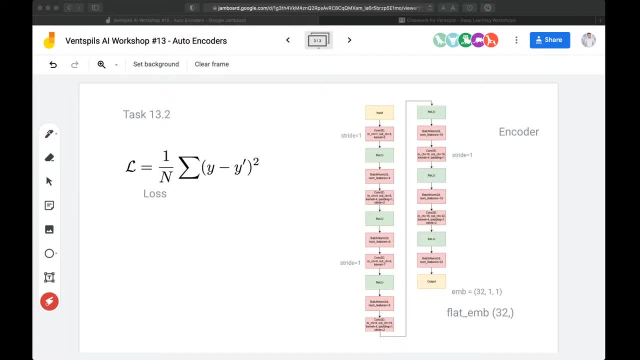 course, the loss will be completely off because you're understand why it's completely off. Probably Christopher should be able to understand why the loss is completely off right now. So let me look. I will start showing some stuff. I see that some people are struggling with. 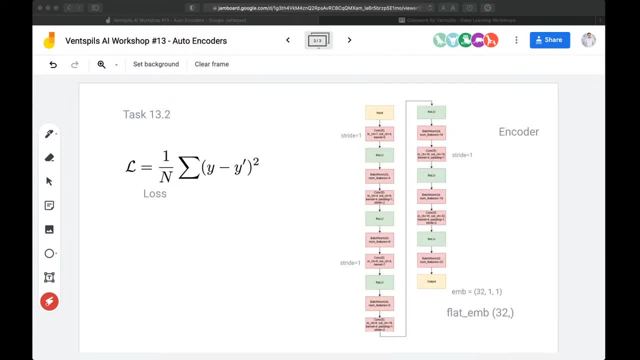 the loss function, that you should not be struggling with it actually. but it's fine. It's better that you try not just not give up, you know. So the error that Lee shared this is quite normal, you know, like it's expected. 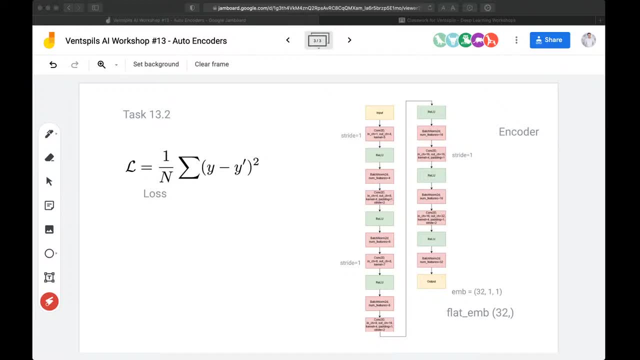 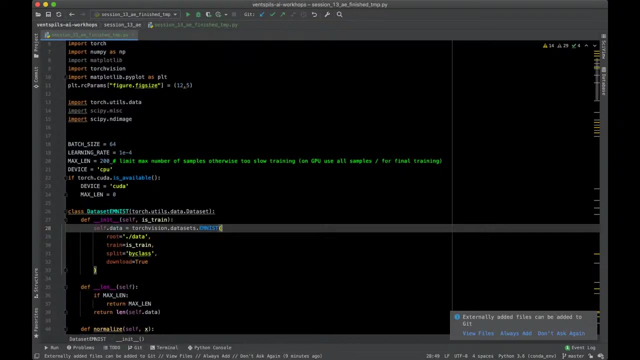 because it means that you're trying to select one item from a vector of losses. but basically it will never work like that, Okay, so let's start doing by this second part. So here I will zoom in a little bit. Okay, it's something, not. 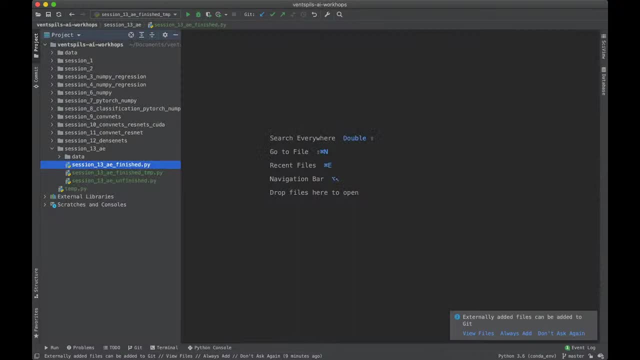 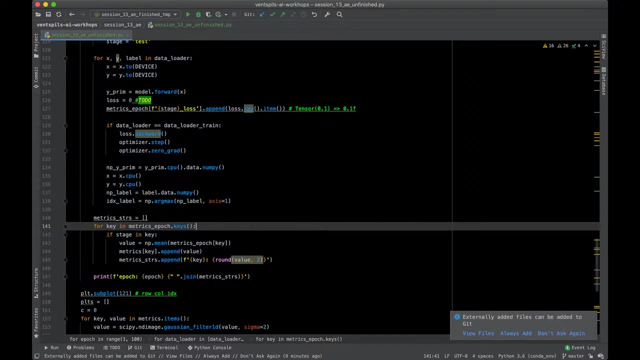 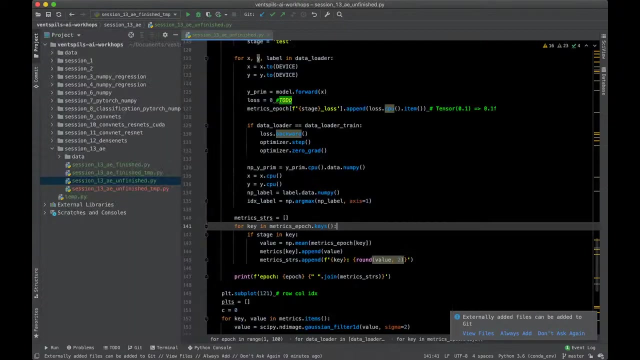 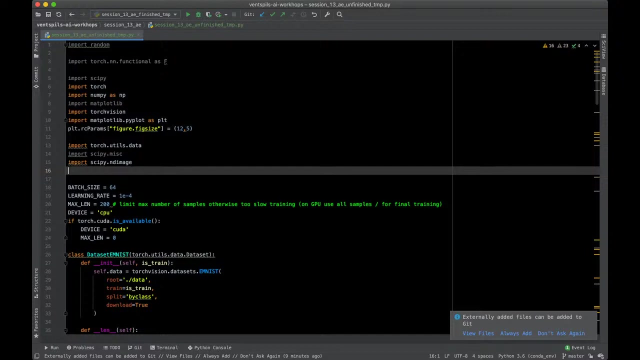 really what I was expecting: Unfinished right. File save as this as tmp, so just that I have another file here, Right, Okay, cool, We have it already. Lee submitted. That's great, Okay, So I will check that a little. 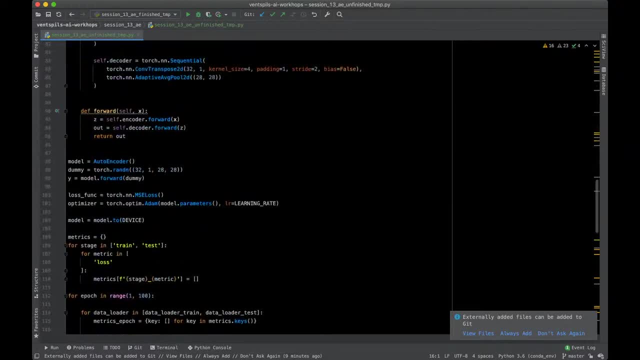 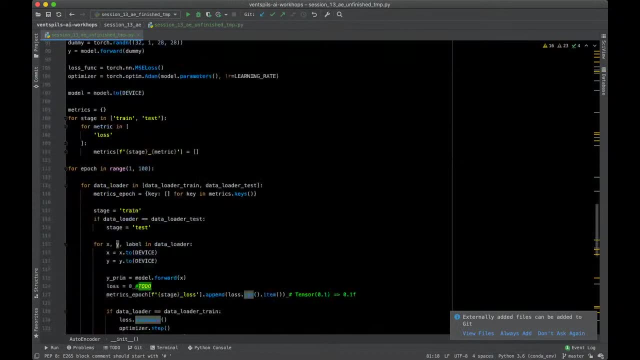 bit later, but that's a good progress that you are able to do this now. So now- and I will try to complete this part- So some people are struggling with the loss. That's really strange, because this is mean square error. So that means that you. 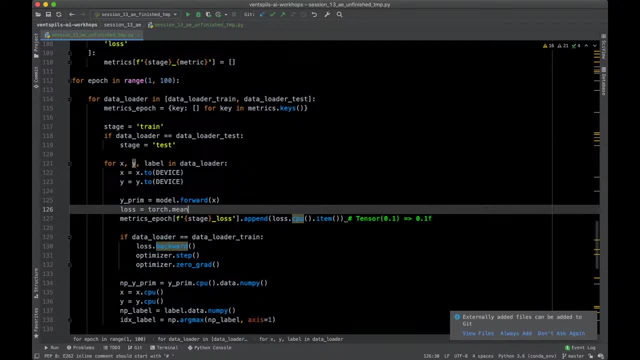 recall mean. So that is the part of the equation that's very easy. So then the next part of the equation is the y minus the y. So that's the part of the equation that's very easy. So y minus y, prim. 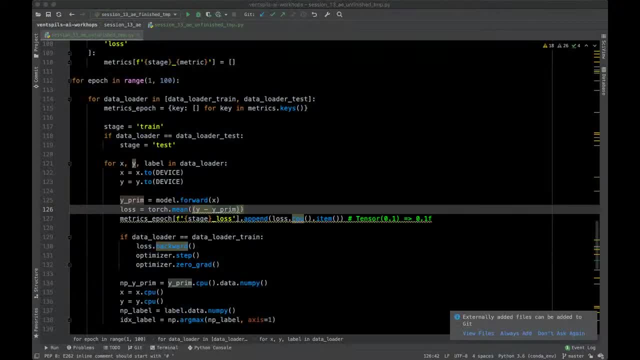 Right. So we have also that Kilo submitted, that great. So here we squared it Right. So this is very simple stuff. here We use the very basic mean square error, like one of the first things that we did, Like we even made the. 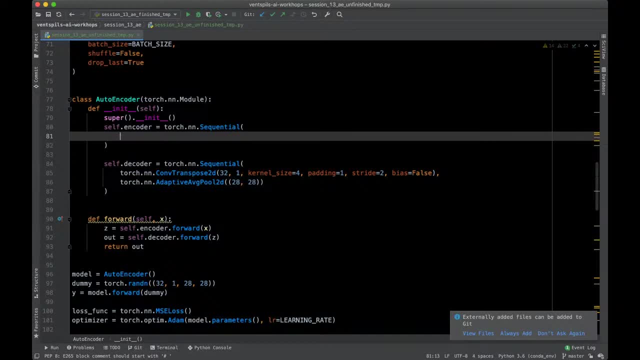 derivatives by hand for that. So here let's write all of this stuck with the encoder. So convolution, the in channels is one, out channels is four, the kernel. so it should work without errors, if I may say. So. if you have errors, then it basically means that there is something wrong with 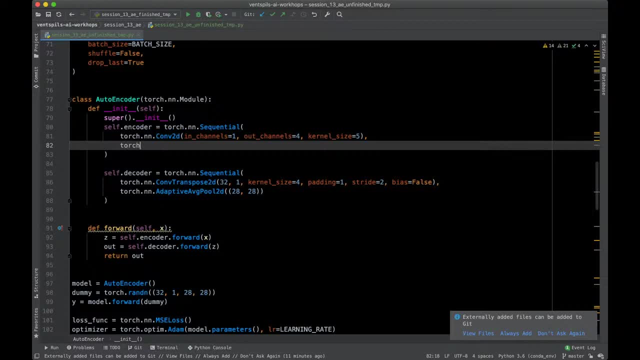 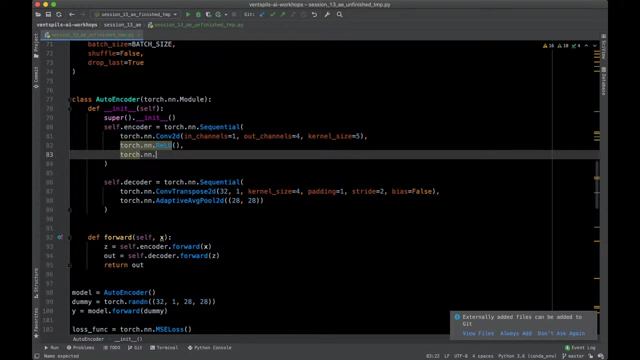 this code with your code, So, rel, just so that it would be more fun, maybe? no, I will just stick with the task. So, torch, and so I will do proper architecture for you at home. So num features, for so now we have a. 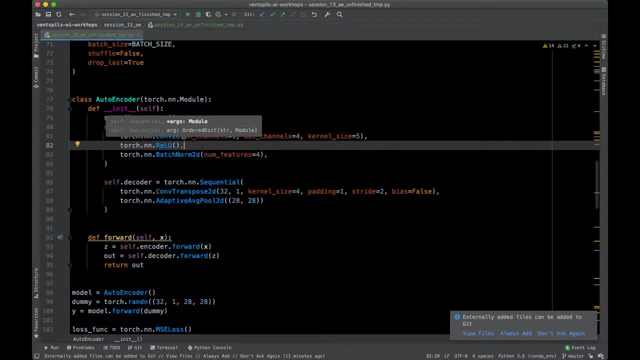 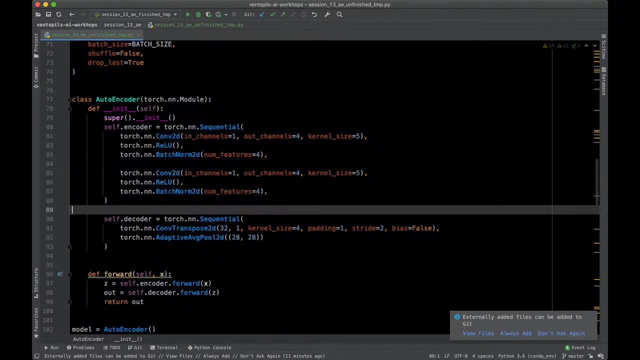 small block That's kind of repeated so I can try to just copy that part like this, this thing. So now this is repeated again for the next part. So for the next part, this is 4 in channels, of course, 8 out channels. kernel size 4, stride 2, padding. 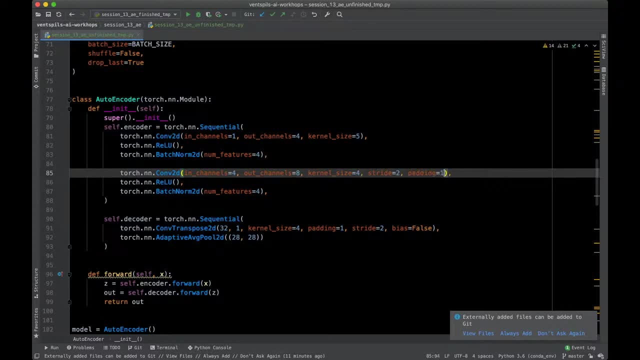 So if I would be not nice, I would ask you to calculate all of this stuff and also the dimensionality of the of the embedding at the bottom. So you already know how to do this. but in this case we already have all of the numbers ready for you. You just need to. 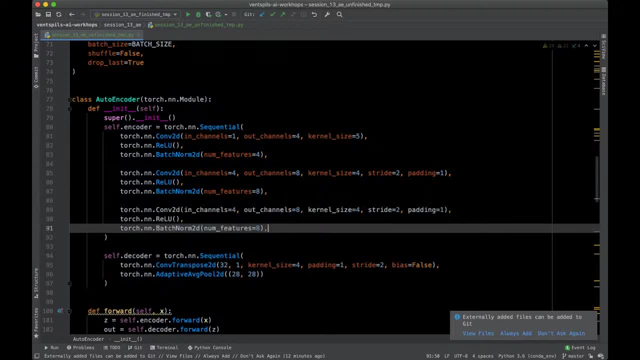 place them in. So here the next part, the 8,. so this one is not changing the channel, it is just working on the width and height so that the stride is 8, and 8 and 6 are neutral and 7 are non- Moskva Serving. really well that you see. not bad for future. more them values, so that the stride is between 8 and 9, same way it should be東西 как отмéroczки, siis tons нераюкорачары. 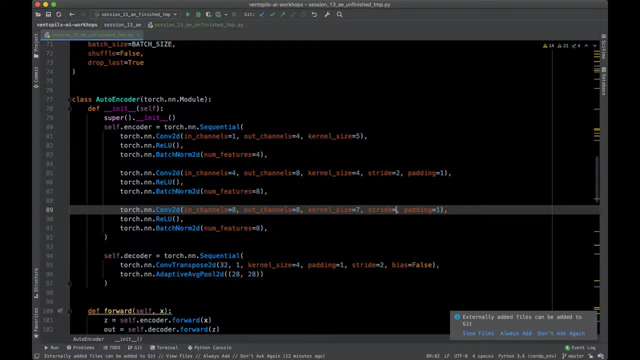 left, as, by the way, in this one I left out. so the stride by default is 1 and padding by default is 0, padding 0, so here the stride will be 1, the padding will be 0, like that. then the output will be 8, then the next. 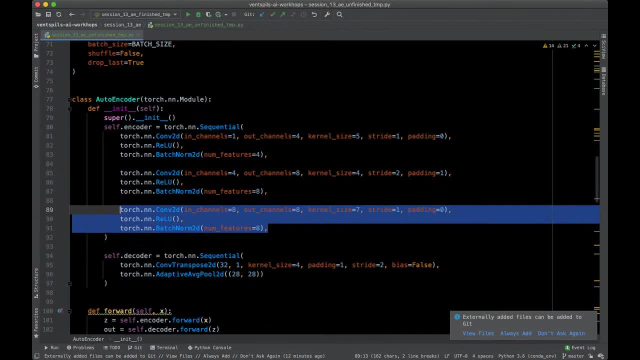 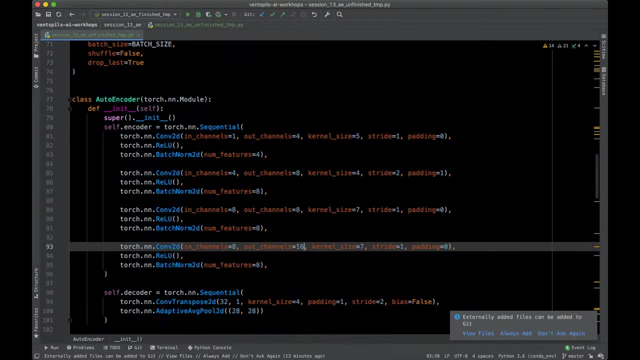 iteration. so we'll have 16,- oh sorry, 8 to 16, then we'll have the 4 kernel size, then the stride will be again 2,, so we're reducing it by. so we're reducing it twice, but not really exactly, because we have padding of 1, but still fine. so 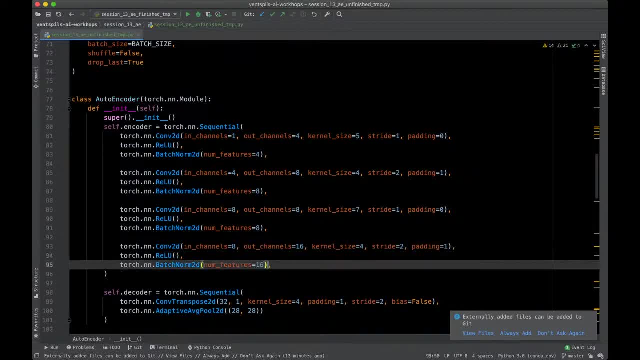 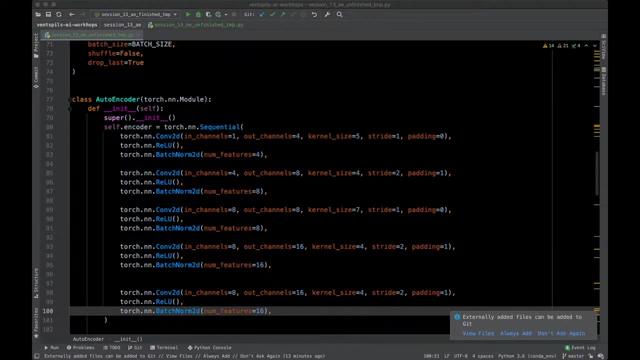 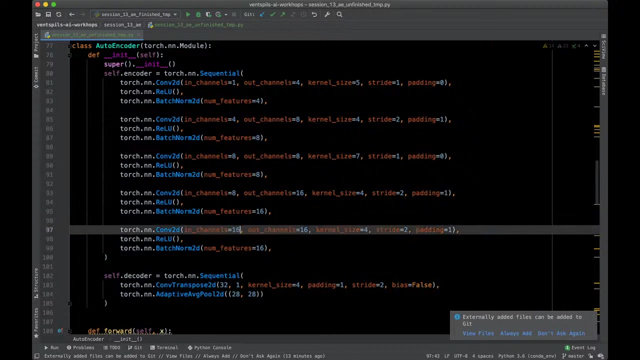 then 16, so it's not really like perfect model, but it will work so, and then, from the 16, we have again the one layer where we just don't change this size. so 16, 4, stride 1, padding 1, hopefully, yeah, like that. so, and then, I guess, the 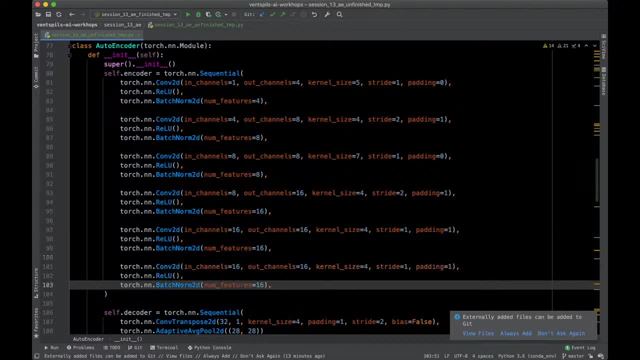 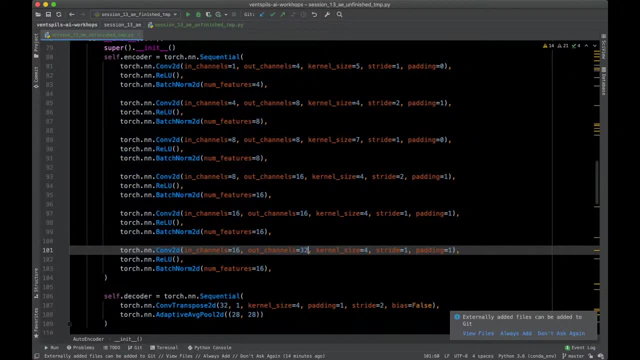 last one. the last one will be 6 to 32,, 16 to 32, 32,, then 4, 2, 1,, 4, 2, 1, and if this is correct, then by running it it should not crash. if it's not correct, there is. 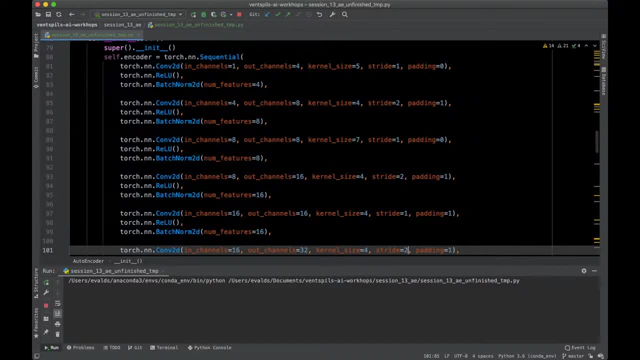 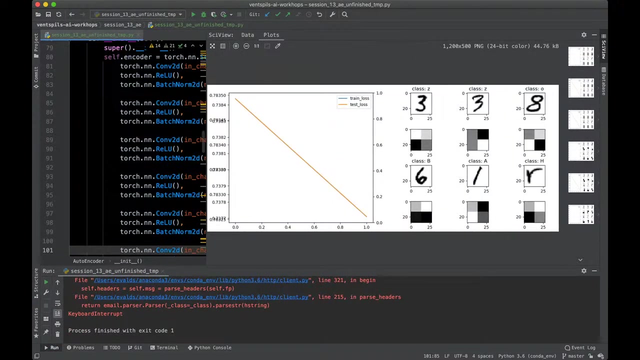 going to be error. so if I run it, okay, it's not crashing, cool. and here is also the thing that I was talking to you: that the class name here the B, A, H, so on. so those are wrong. so the classes in the data set, the labels. 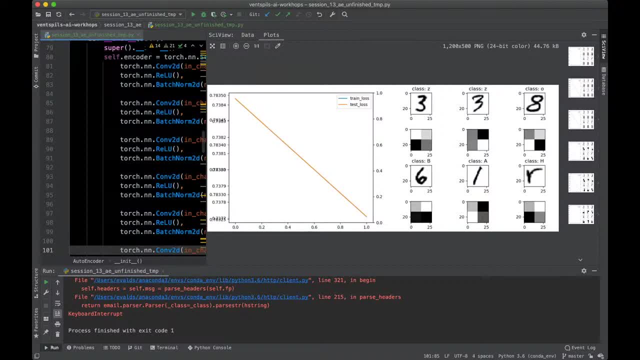 are somehow mixed up. I will for the homework. hopefully will find the correct labels for this data set. I think this is a bug in the torch vision, so, but that's a small issue basically. and then you see that the decoder is really dumb and it just creates some random stuff, basically. 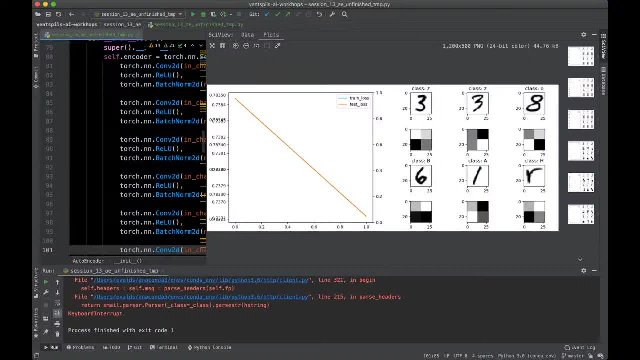 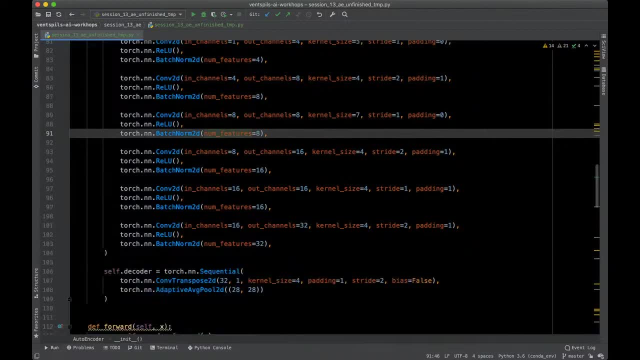 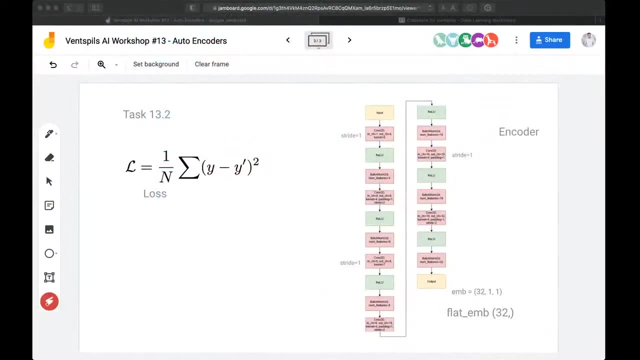 because we have. we don't have proper decoder yet, so we need to create a proper decoder. this is going to be the next task for creating the proper decoder, so I will briefly open the task in the Jamboard- I mean in the classroom- but before that I will explain what to do. 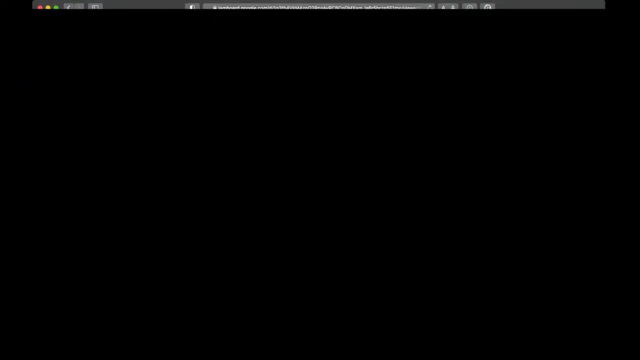 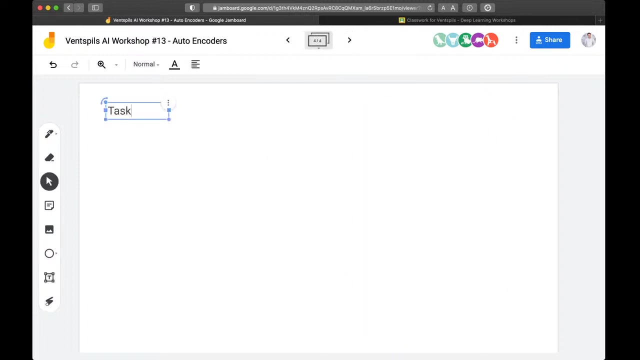 so if you go, then there's going to be the task 13.3,, so task 13.3, so you will need to do two things. so, first thing, regards to decoder, of course the decoder. so with the decoder, it will not, it will be I. 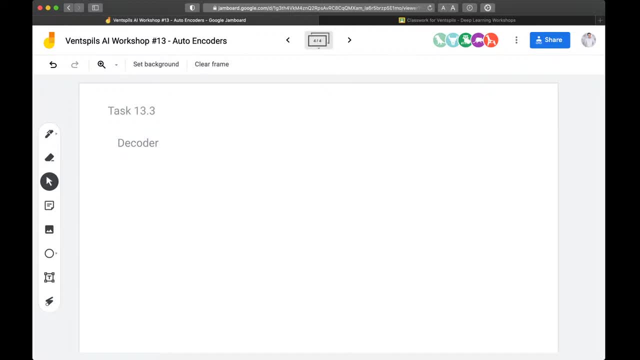 think the first time when we start to use the transposed convolutions or some kind of generative model type of things. so the transposed convolutions are have also the equation for the output dimensions. so if you remember, there was one equation for. 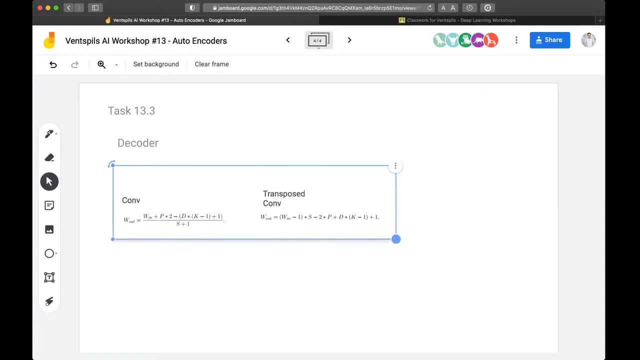 the convolutions. here the D is dilation, so dilation is in this case it's always one. so let me also type in: D is dilation. so I will double check if I'm not misspelling this name: dilation, convolution. oh sorry, I am misspelling it. 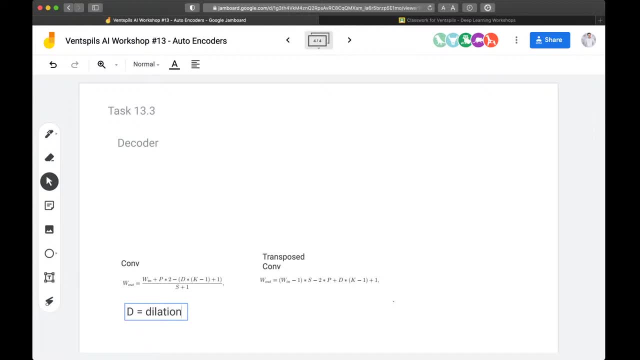 dilation, sorry. so dilation, right. so that is basically just to visually maybe explain so that your let me show. so when dilation is one, then your kernel looks like this: when dilation is two, then your kernel will look like this: 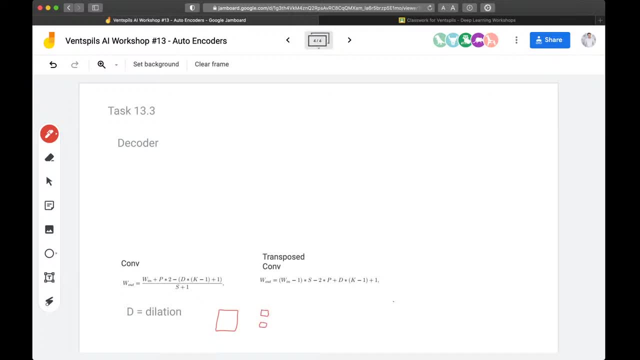 for example, so it can have some spaces in between, but in this case we will not use really dilation. dilation is you are used in some specific models, but basically I'm just writing it here because it's in the equation and you. 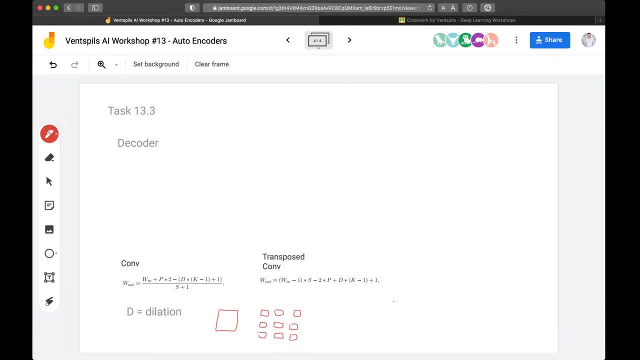 should know this name because it appears time to time in some papers and stuff like that. so here the dilation is one. so this is equation for the transposed convolutions. the dilation is one for this type of kernel and the next thing, that for the 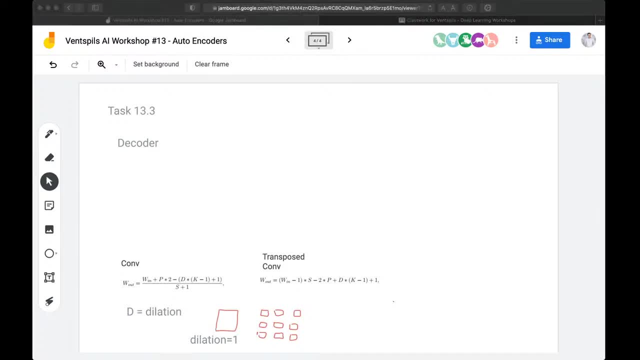 transposed convolutions. that will help to understand how they work is the following image. so I think in the PyTorch it was called. it is called conv transpose 2D so I will also write down that one, so the actual name of the function. 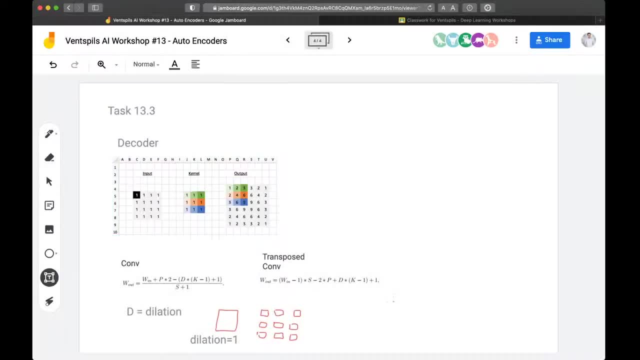 is conv, transpose 2D and what it does. so you have input image here and you have kernel here with the code marked colors, and then you see that it calculates the values with regards to kernel and place that on the larger. 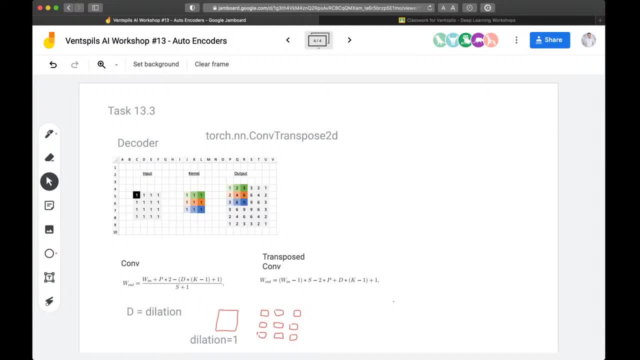 image by the method as displayed here, but basically so it's kind of it's just using the same value from the one pixel and then doing all those dot products and summation from that one pixel to create the larger image. so it's. 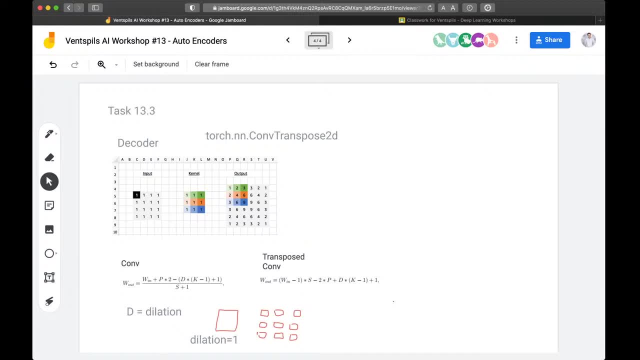 kind of the opposite direction as the convolution. but yeah, so you should not actually spend too much time, I would say, researching all sorts of things with transposed convolutions, because in modern models they actually don't use anymore those, they just upscale and use the. 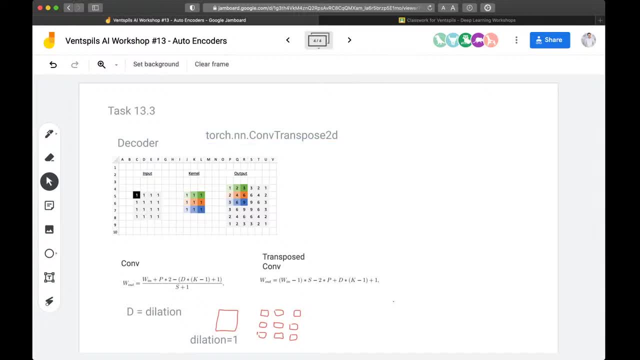 convolutions that don't change the width and height size, but still it's. this is something that is useful to know, and the other part that you will need to implement in this model so is the denoising. so I mean the, I mean the noise and adding the noise. so that's why actually in, in. 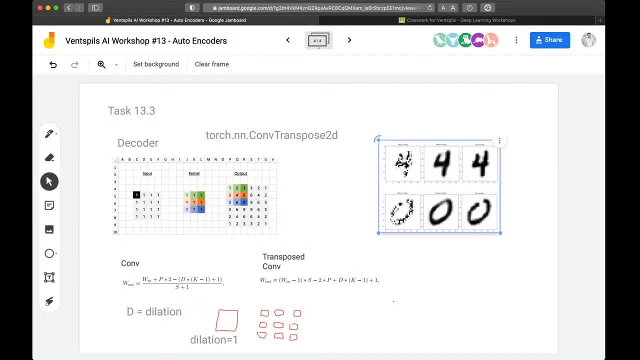 your data loader. I specifically created three types of inputs. there is a, there is a X, right, so then it. then you will have the Y here, right, and this is going to be the last one. it's going to be Y prim, so. so I want you to create first the decoder. I will give you architecture in a moment, and 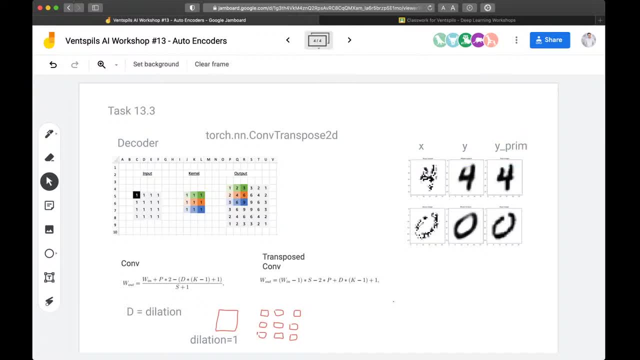 I want also you to create the noisy data set. basically, Vasili, you will just add the noise input and this will be called the denoising autoencoder: a denoising autoencoder, denoising autoencoder, denoising autoencoder. If you read scientific literature, it says that denoising autoencoders. 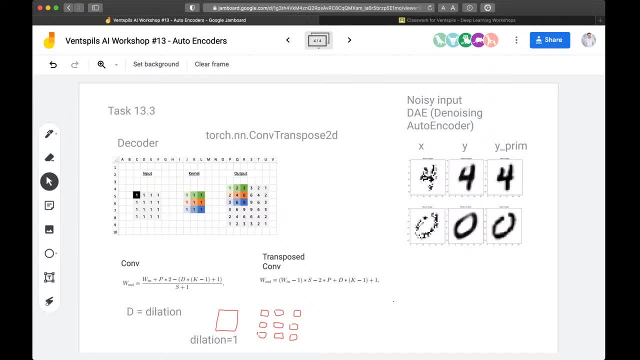 perform much better than simple autoencoders. So you have this part as well. Okay, so I will add this to the Jamboard, to the Google Classroom, sorry. So I see five submissions of the previous task. That is excellent. Almost everybody that is attending this session is able to do this. This is: 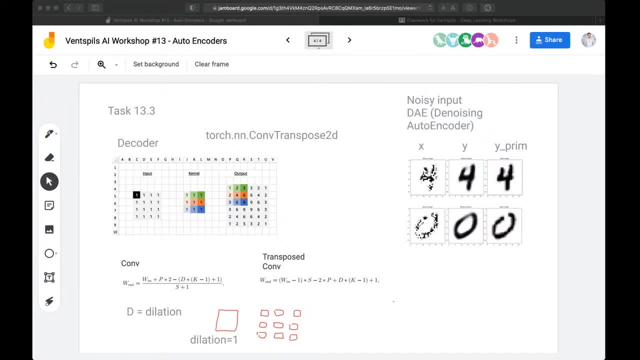 great. So now you already start, you can start working on the next task, basically. So this is going to be 13.3.. The decoder: decoder plus the noisy input- noisy input. So I will add the architecture. So this: you will use the same template as from the previous task. You don't need to create a new. 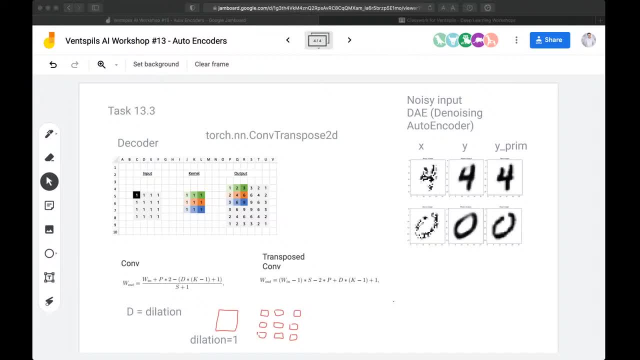 template: right, So you use the previous task template and just complete the decoder part. So I'm dropping it in and adding to the topic. topic of autoencoders. So it should be live now In the Google Classroom, the task. 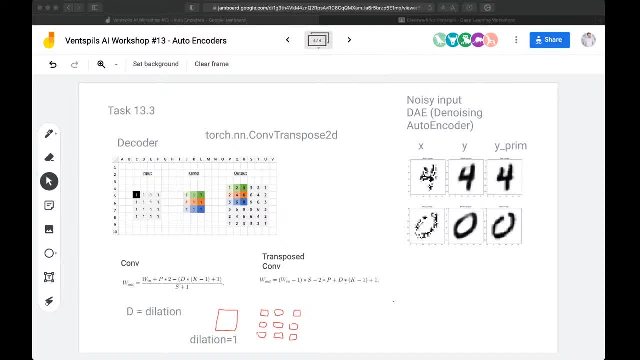 so I will maybe add a little bit more details. So implement the decoder using model schematics And also implement data set X as noisy using some kind of random. So basically, the problem is that we have one pixel here, So let's say that. let's say 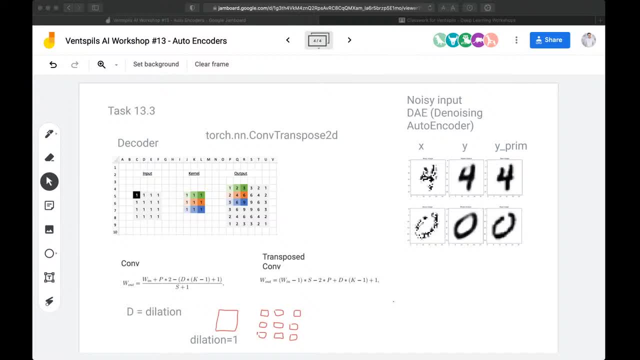 you have a pixel here and then you get that zero pixel. Let's say you have a pixel here and then the random, random under 0.5, then set it as zero pixel value. pixel value. I will also copy this this one here. So if you have questions, type in the the chat, I will just look at in a second. 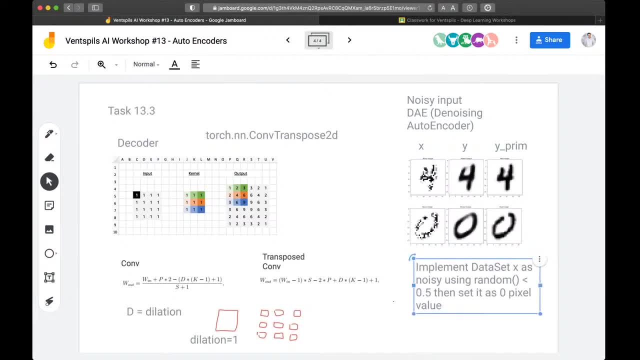 So basically, if the random for the pixel is under 0.5, then set it as zero pixel and it should be at the top, So that way you're not seeing that it is a comma, You're not seeing the other up. 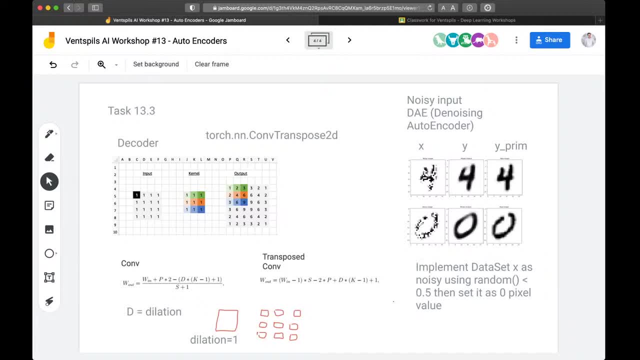 So if it is a comma and so on, then make sure you have that zero pixel value, And then again you're not seeing that it is a개 all and you're not seeing whether or not the pixel and it will create this kind of noise here. So this is what you need to. 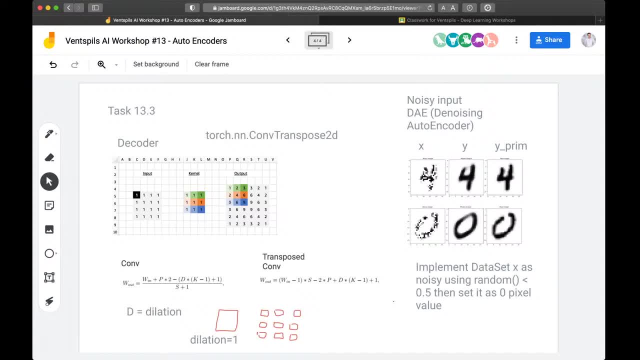 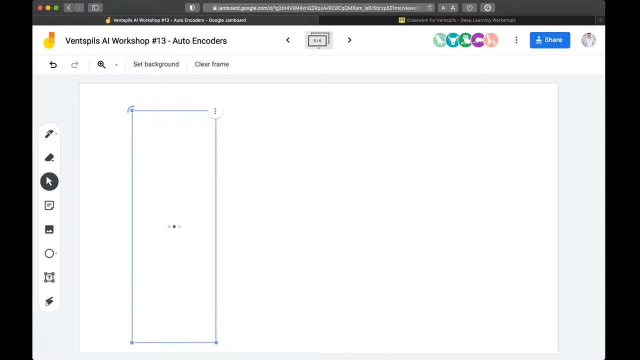 do and the actual model that you need to make. I will add that as well. So in the slide 5, let's have the model. So this is the model in slide 5, decoder and yeah. so so the idea is that the embedding in the middle part either by Euclidean or by 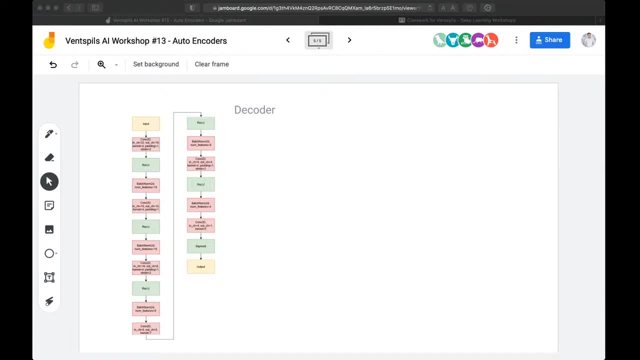 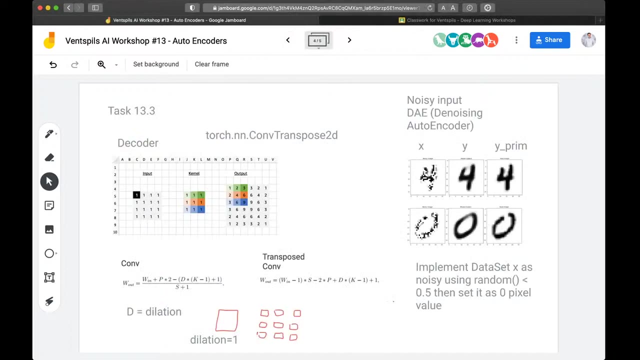 cosine distances will- some will kind of like have the the ability to cluster together by similar images. so and it's, it's done completely in an unsupervised manner, so we're not telling anything in regards to labels and stuff. So I hope the task is clear, so maybe let's check. 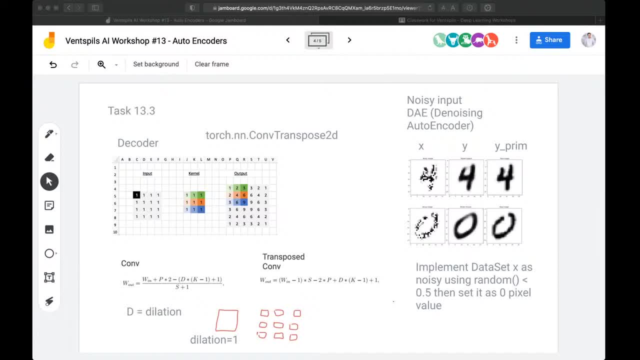 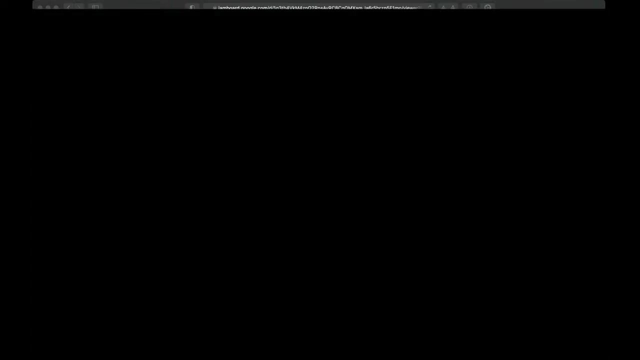 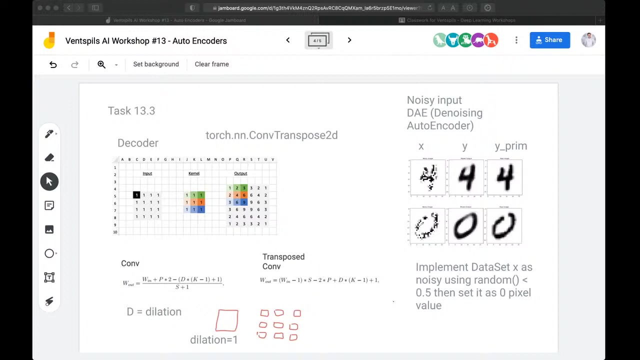 if the task is clear. So I will ask: is the task understandable? If you're sure, a table, long, long, long înt long generative part is something that you will also see in UNETs and some other types of models that I know that, for example, Kirill and Robert and Kirill and Christopher's should, should be able. 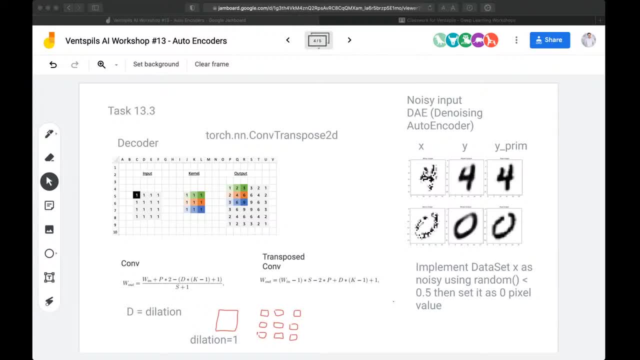 to work with the UNETs very soon, so so this is a first step towards UNETs, basically. so I see one plus with regards to tasks. so please try to do this task and submit the results, and if you submit results, you will start seeing cool stuff happening and also you can run this code. 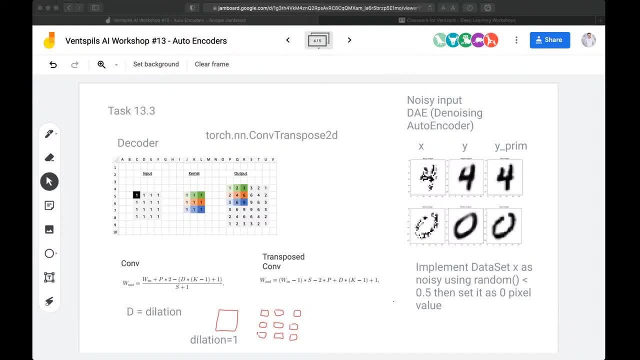 directly on Google Colab and then you will see even cooler stuff. but you will need also to find the hyper parameters, probably because the default hyper parameters are never the optimal hyper parameters. you I didn't quite understand about the second part, but about, so the second part? 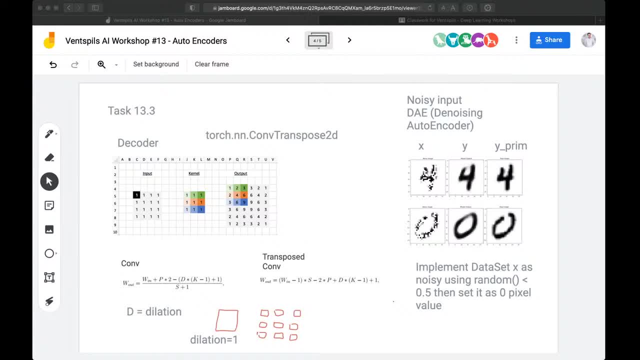 the. so this is a transposed convolutions, so the transport convolutions by the nature increase the size of the input. width and height. what I mean by hyper parameters. okay, so with a height. so this is a width and height of the input and if you see the width and height of the output, depending on the stride and the the. 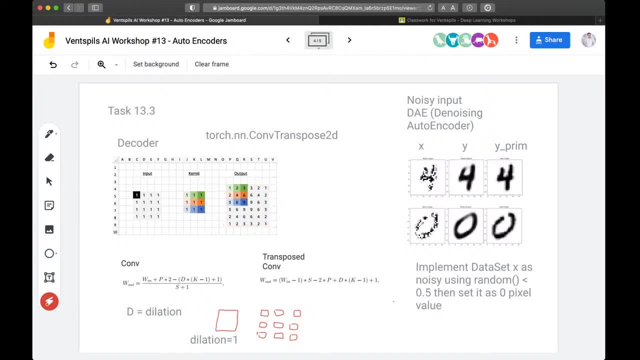 kernel is much larger and you can see that also by this equation- and this is basically kind of similar operation- than with the kernel operation. that was it in the convolution for reducing the size. now it's just like for increasing the size. that that is one part and you can implement that using basically you. 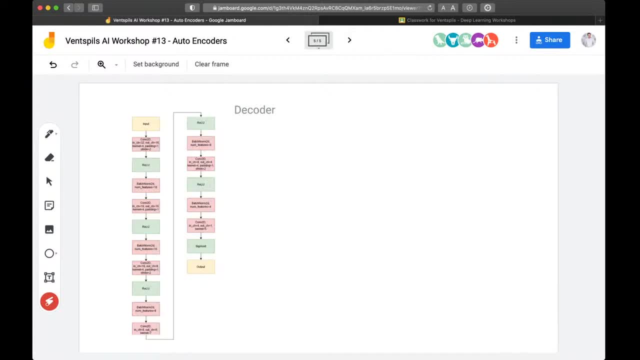 have here, where you have these? I hope, yeah, so convolution to D. so these are, all of these are transposed, convolutions, so transposed. so it's actually con transpose D participants, you can use params. and with regards to the hyper parameters, the hyper parameters, let me 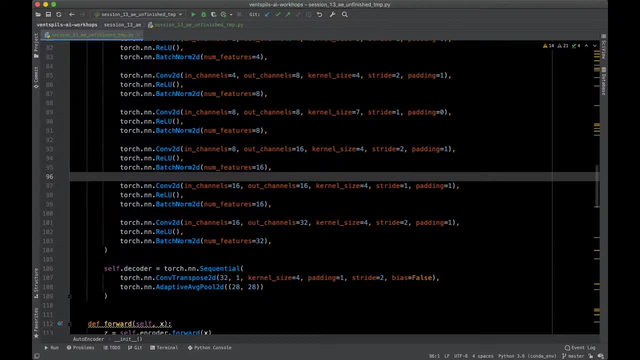 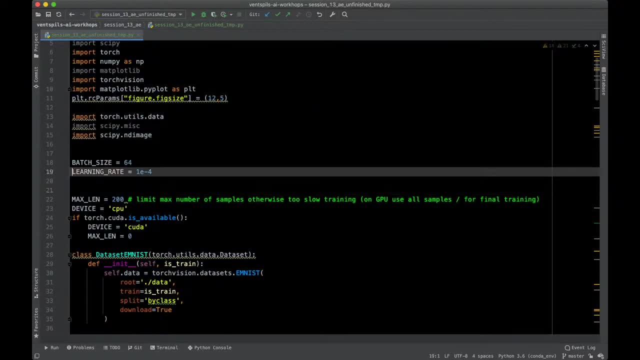 show you is: are the DA actually the learning rate, the batch size and stuff like that? so, and also the depth of the model, for example, there are many high parameters in deep learning. so here you have some of the two basic ones: the model to work great, without exploring and trying to find these like which. 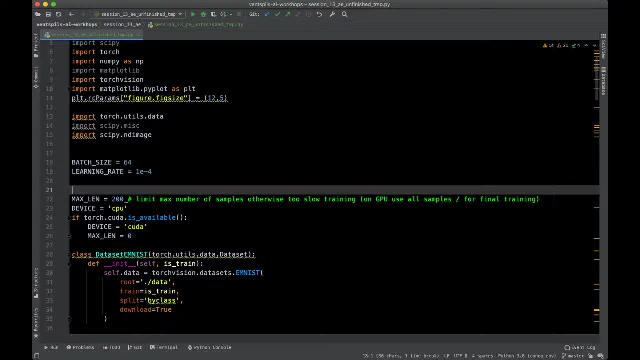 works the best. so usually you would do the grid search, you would try, let's say, e-3,, e-4,, e-5, you would try this one: 32,, 16,, 8 and so on, and all sorts of combinations. the one thing that there is a correlation, so I can give you that. 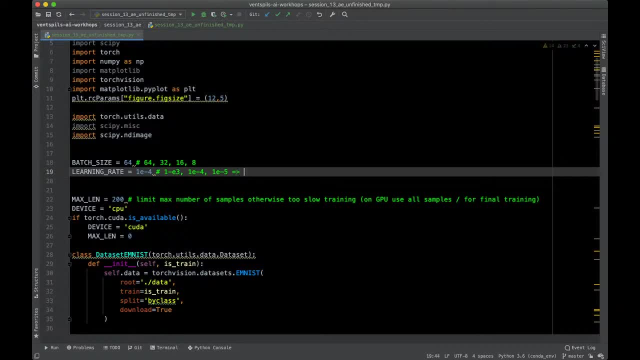 correlation so that usually the larger the batch size, the larger learning rate, like that and the. there is also one big issue. so usually if you have so on another task, so if you have, if you have the batch norm, you need at least 32 plus samples. so this is a big problem when 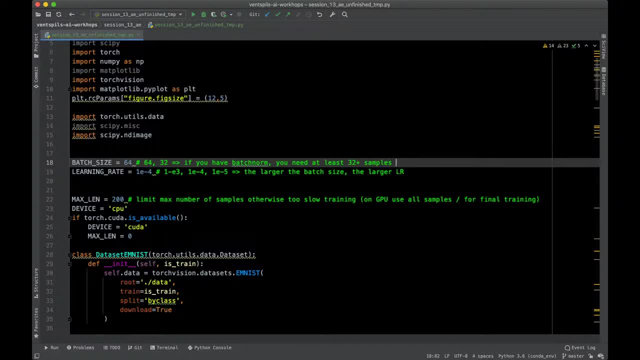 you have, let's say, large images of, of inputs you it would not fit in GPU to have 32 images and this will be a big problem. that's why in the modern models you don't use batch norm, you use group norm and basically that's the same as. 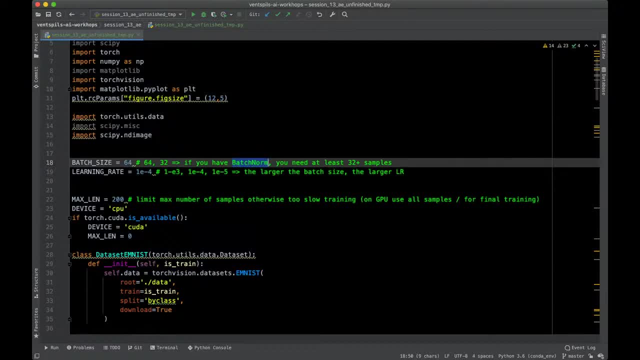 layer norm and instance norm. I will briefly touch that by the end of this, this workshop, and I will also give you to work with that in the homework. so what I'm trying to tell is that the learning rate, batch size, the depth of the model, the model of the loss function. 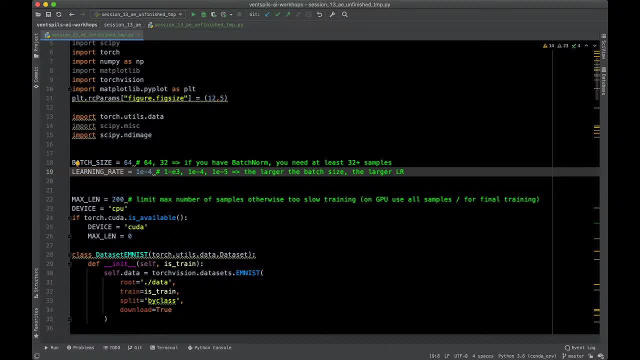 even the optimizer. all of these things are hyper parameters and you cannot rely with one set and say that this will be the best results. you need to file, research them. so yeah, I will wait a little bit and then I will show you how to do it in the next video. 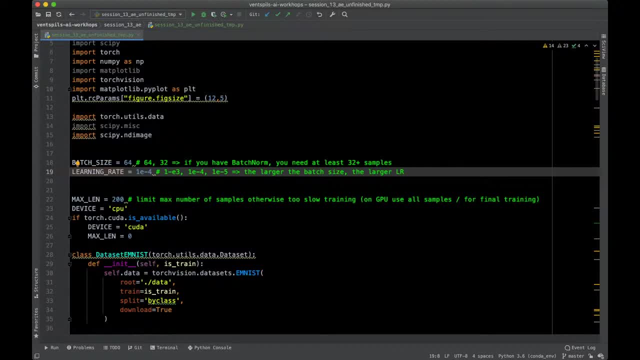 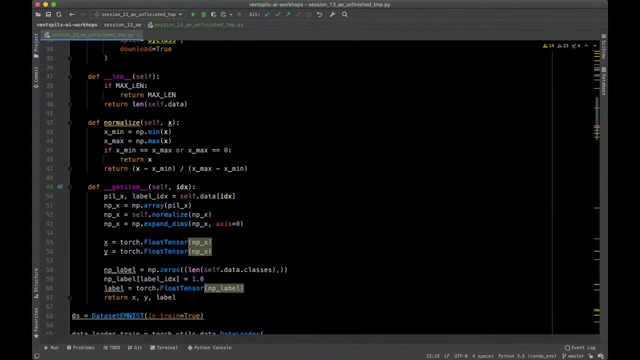 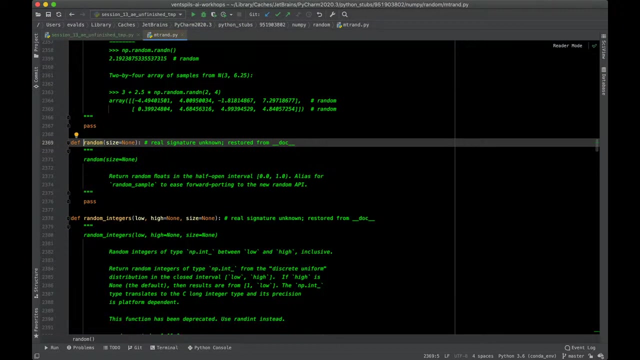 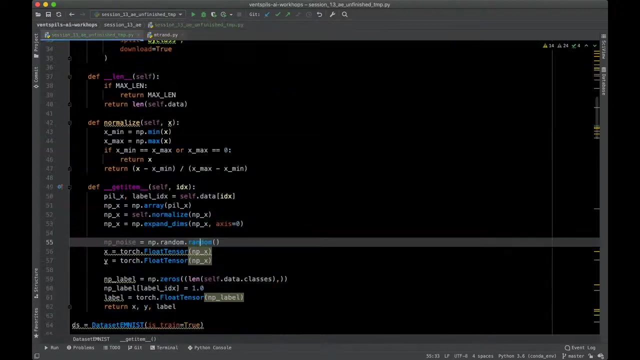 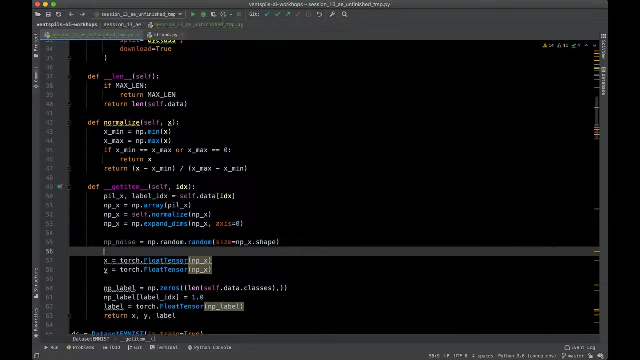 bit with regards to the task. so hopefully you're able to finish this task and meanwhile I will prepare this. this last part regarding the normalizations, you can see that I'm using the, the, some for loops, but you can. you can do for loops if you want. so here under the 0.5 you'll set this as a 0, otherwise we'll use the. 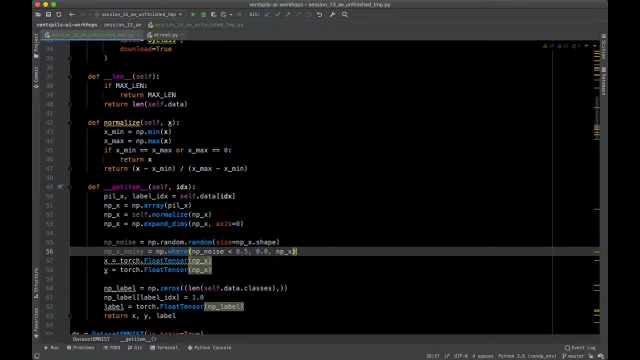 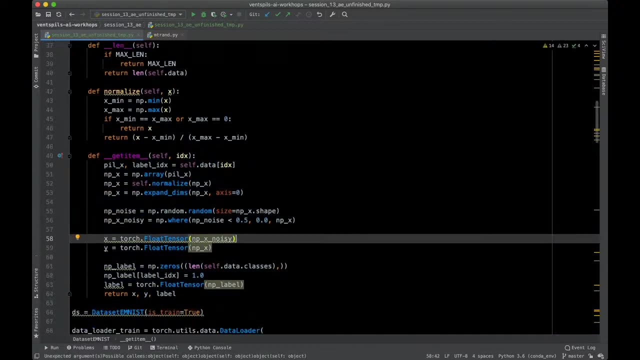 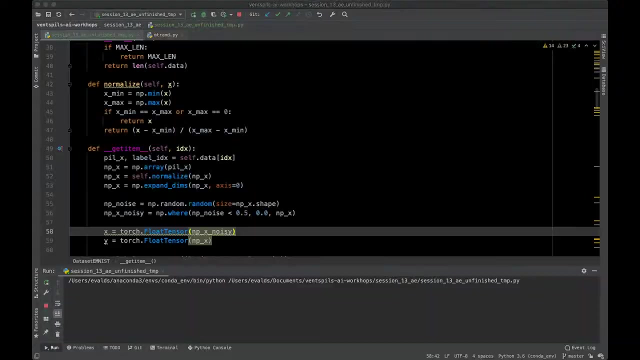 NPX here and now we have the NPX noisy ready matrix here. so that's, that's ready. you can use that. that's for the X, that's great. so if I run it and just double check that there is no bugs to see, great kernel size can't be greater than the actual input size. about the last: 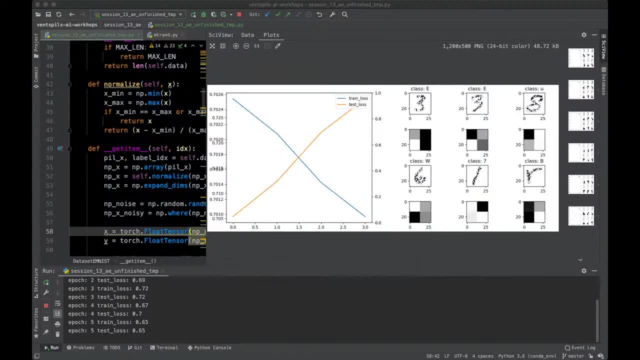 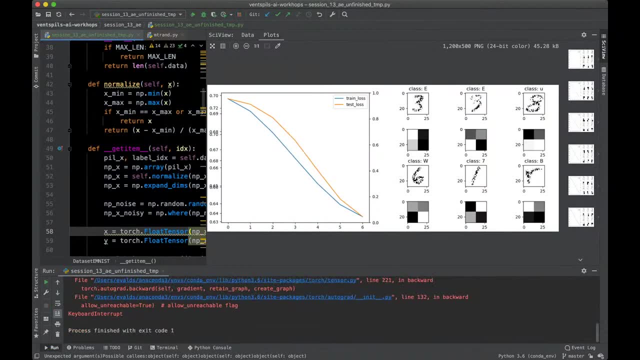 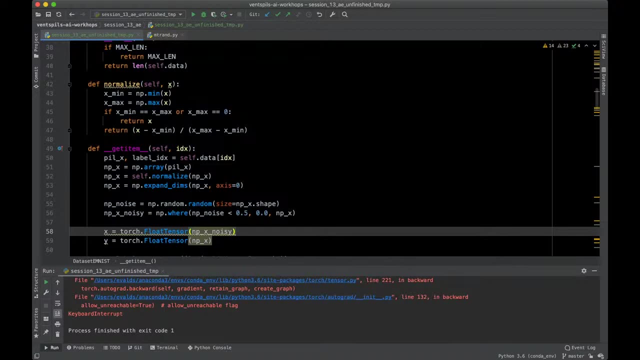 convolution to the: hmm, let's double check, maybe there is some bug. so okay, this one, this worked. so you see that noisy stuff work. so what about the bug? bug, bug, or is there a bug or not? let me check, let me check. so the last convolution is kernel 5. 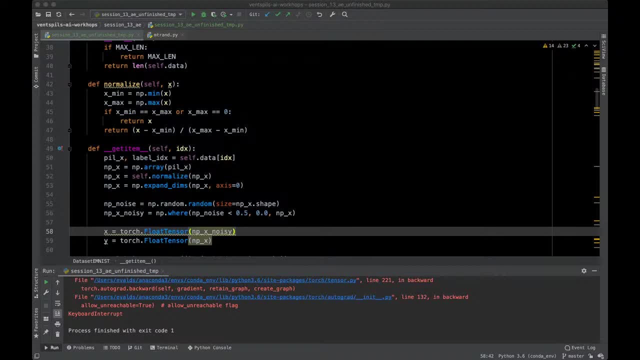 the internals. let's see kernel 4, the next one is kernel 4, the next one kernel 4, the next one is kernel 7. kernel 4, kernel 5, okay, maybe I think there's everts. you might have some like misalignment with with some some part of. 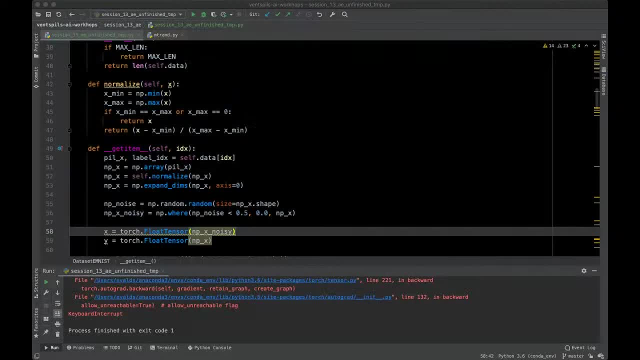 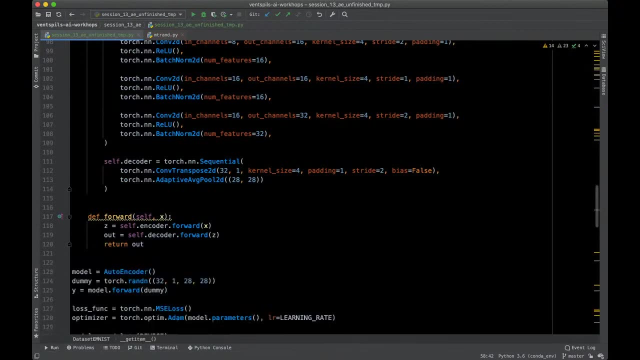 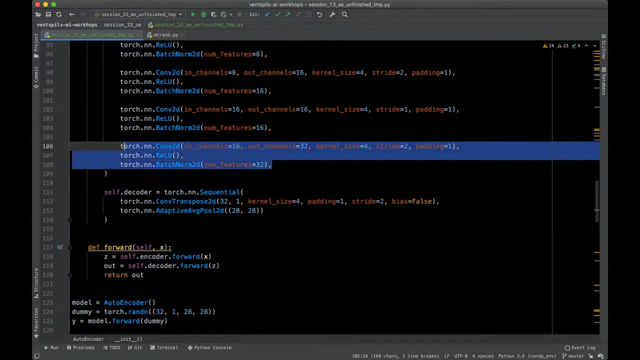 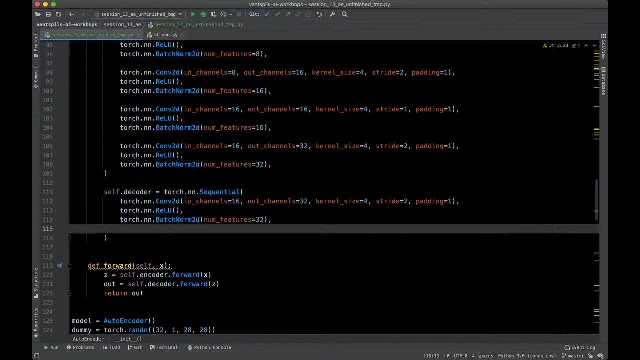 the code probably. so I mean like the, the numbers maybe are missing somewhere, so I will try to do this myself as well and see if I have some problems or not. so basically the, the whole structure looks very similar as before, so, but the only change is that there will be the transpose convolution, so convolution, convolution. 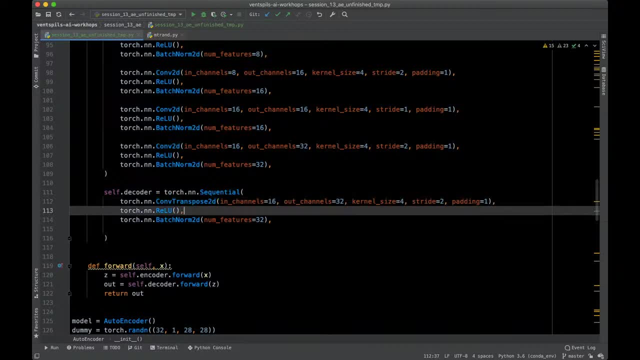 transpose. so the input is then then 32 to 16 and then the kernel is 4: 1. so I think it's like kind of mirror. so for padding 1, stride 2, I think it was kind of mirror stuff, let's see. then there is a. 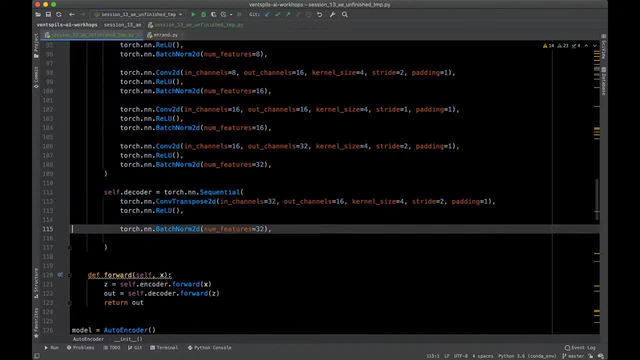 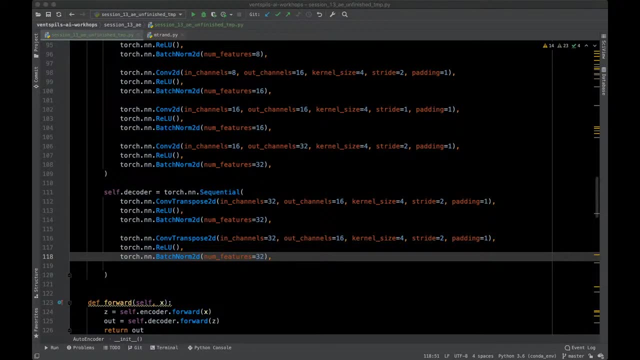 oh okay, I will just follow this closely. so 32, then the next one. the next one is from 16 to 15.. to 16,, 16 to 16, then the 4. so I think it's just a mirror, so you can just copy. 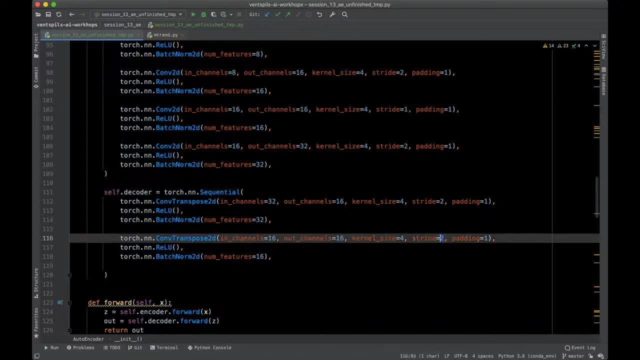 these parts one by one and change to to convolution, transpose convolution, and then it will be fine. I think so. 4 1, 1, yes, yes, yes, padding. only there is a 0. okay, maybe I have had a bug before. let me check. no, the padding. no, it is like. 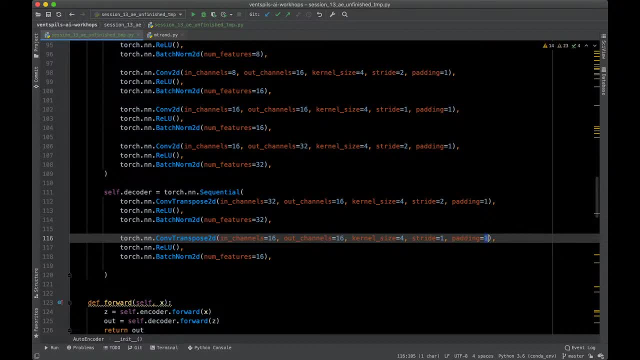 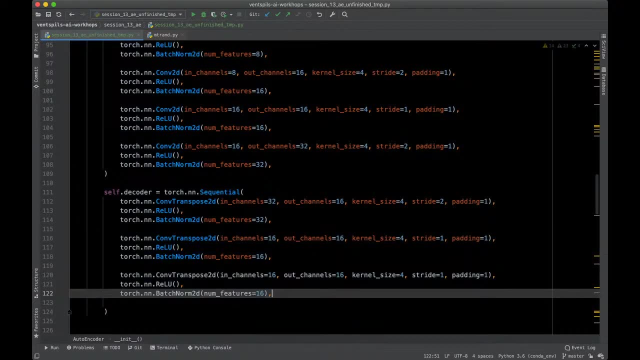 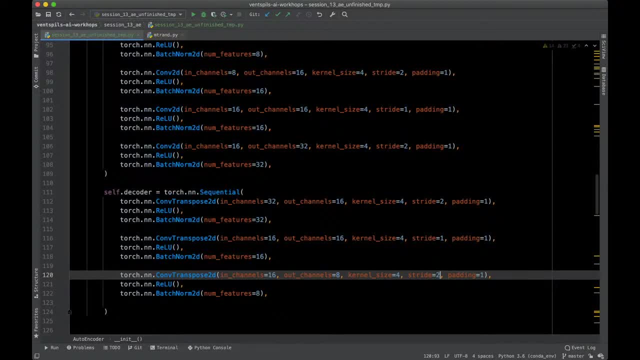 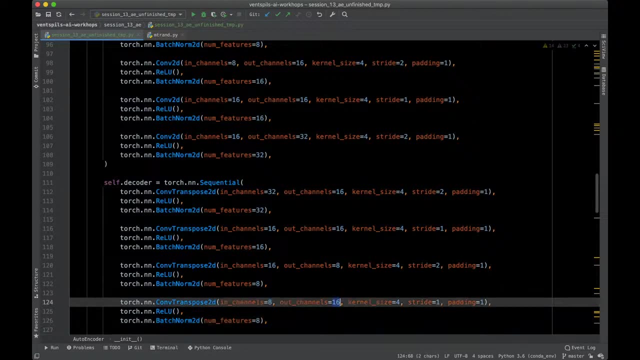 okay, then the next one will not change again. this is going to be the 8 to 8. the channel size will not change: 8 to 8. then from the 8 to 8 there is kernel size 7. this tried one padding, padding 0 only, so let me check if I had that as well up. 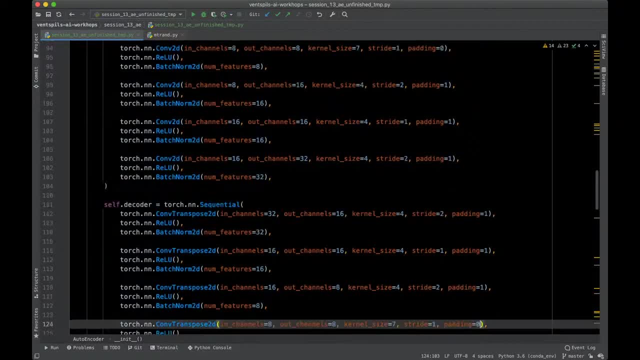 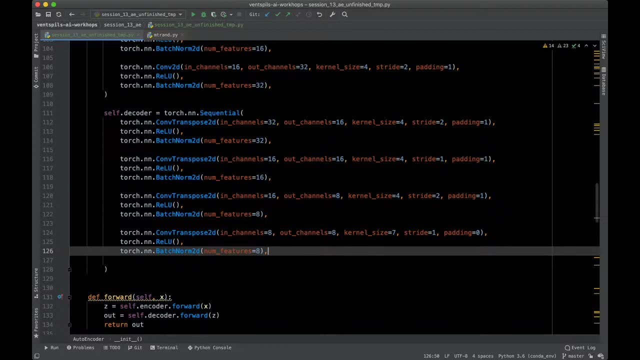 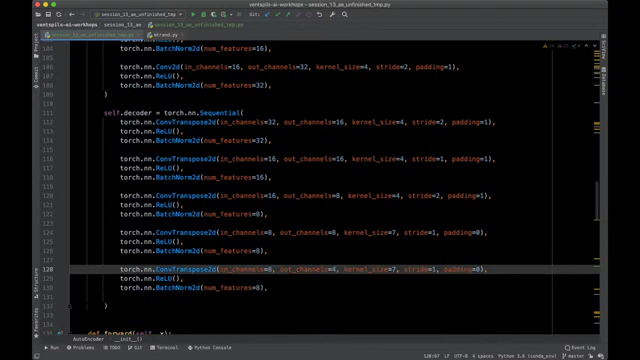 there. yeah, padding 0. cool, that is correct. so it's quite easily to. you can something like mess up something, but still so. then the next one will be from 8 to 4. 8 to 4, then the kernel, so the kernel size will be 4. 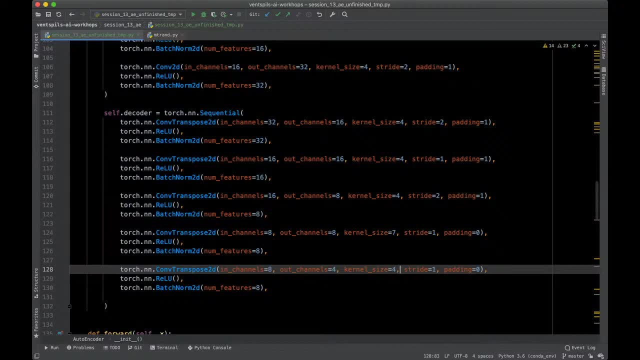 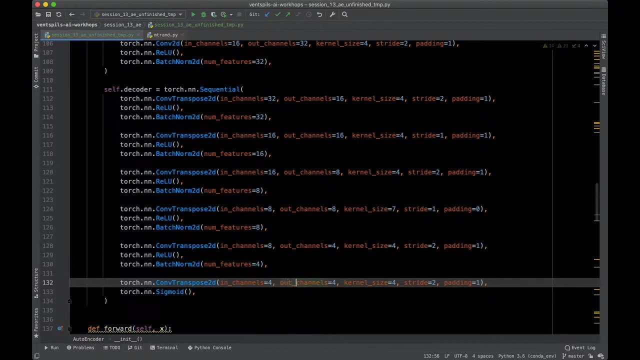 stroke padding 1 and the stride 2, so then the features will be 4. that's right, so that's cool. so then the last two things will be: the here will be sigmoid, because the values of the output will always be from 0 to 1. so 4 to 1. the. 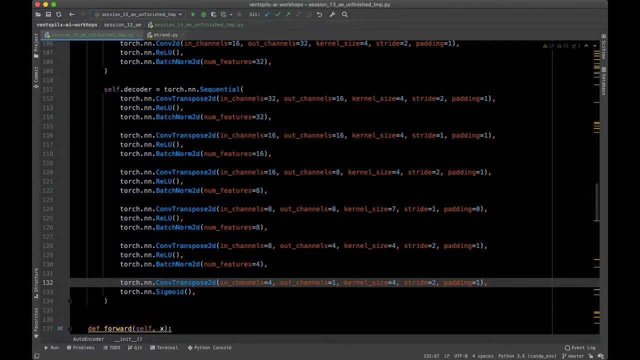 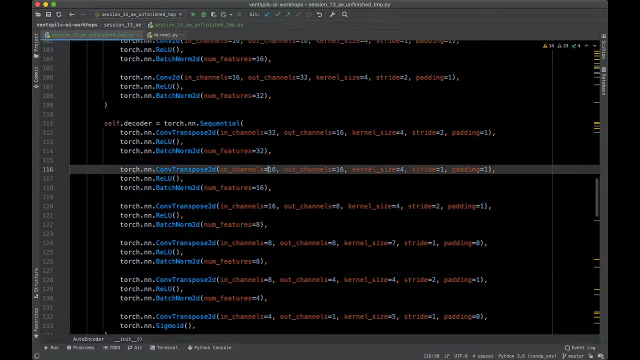 kernel size 5, stride 1, padding 0, like that first batch norm shouldn't be features. no, so there is okay. yeah right, sorry, you're right, you're right, thank you, thank you, thank you, so everything I was looking that here. device room. so yeah, there should be 16, not 32, so that's of. 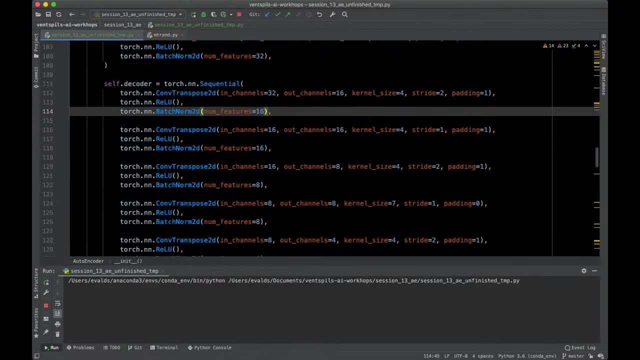 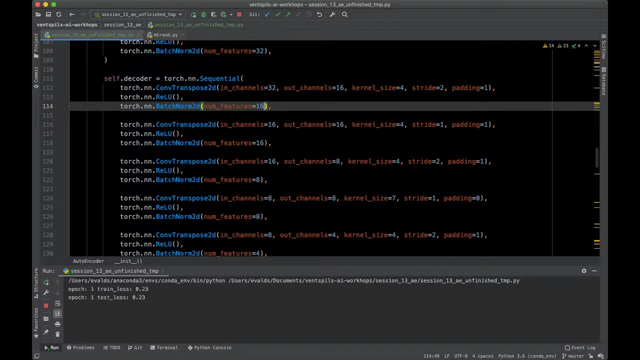 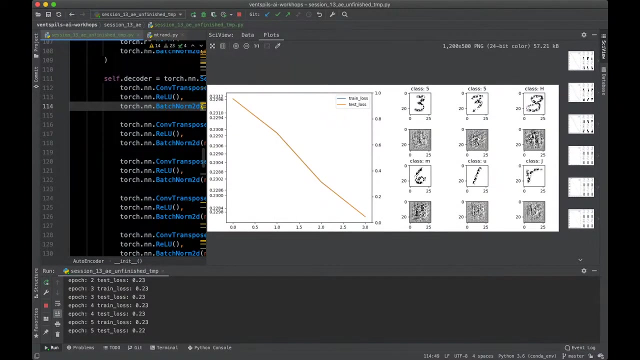 course right. so if I run it, let's see if I don't have bugs, maybe I have- anything could happen. so it works. so there's no bugs. so if you don't, if it does, if it don't work for you, that means that you somehow missed some numbers. something is a little bit messed up. so you see, that is. 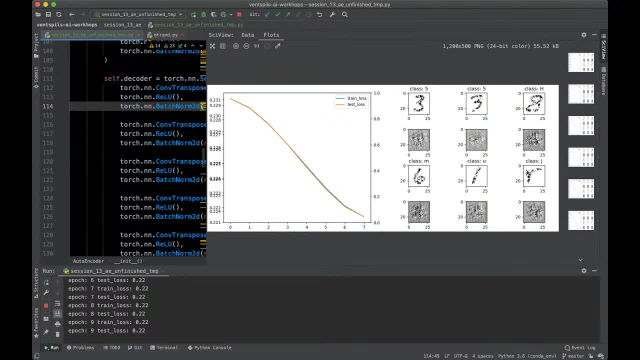 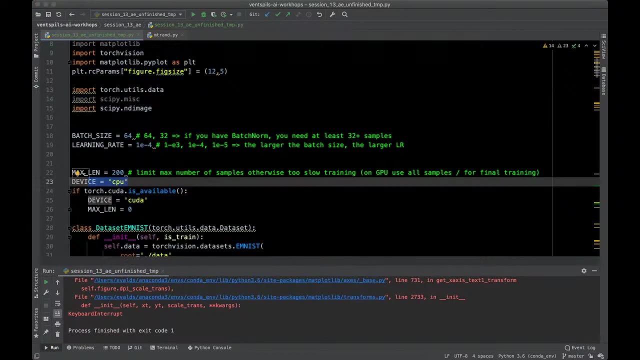 slowly trying to become as those numbers. but of course there are two things go happening here. the one thing that is happening here is that we are running on CPU, right? so see up there, there is a CPU and it. that means that we always only take 200 samples for the, just for the coding. 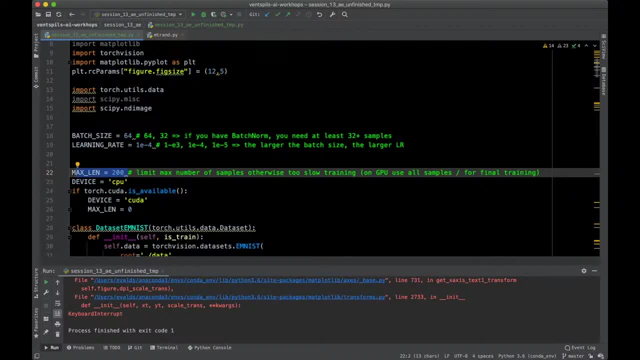 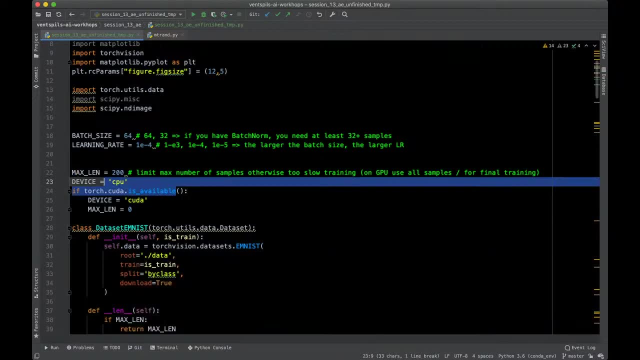 purposes, so that we can see them. but if you would run this one GPU or the Google collab, then we will train with everything and we will slowly to see how these images start to behave, become more like the input images and, at the end, will get the embeddings perfect. so that that is this part called. so hopefully some of 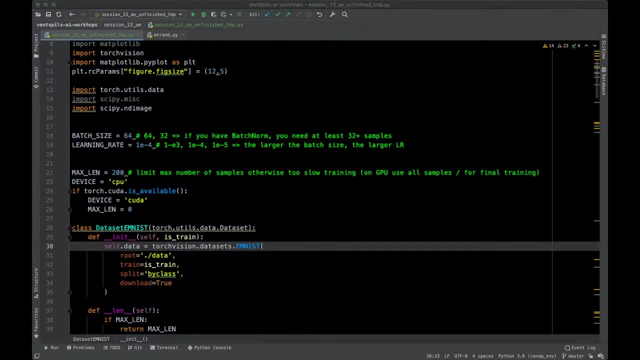 you can finish this yourselves right now. I see that already one person- something that, of course, that's Christopher's- that's great, so I'm just going to recommend my next step. see you guys next week. bye, So let's keep up with the last part of today. 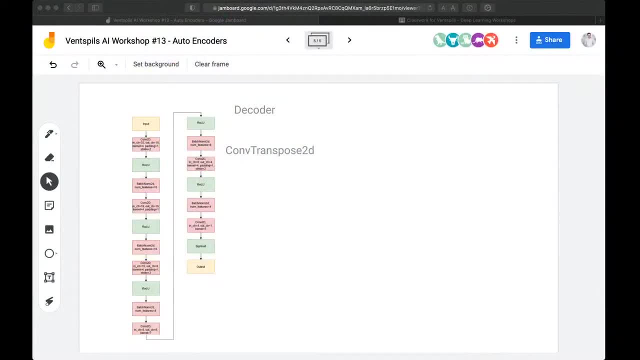 because I need also to run very soon. So homework, I will give you the kind of a little bit state-of-the-art type of autoencoder architecture. So the question was with regards to the batch norms. So the batch norms are not the greatest thing to have. 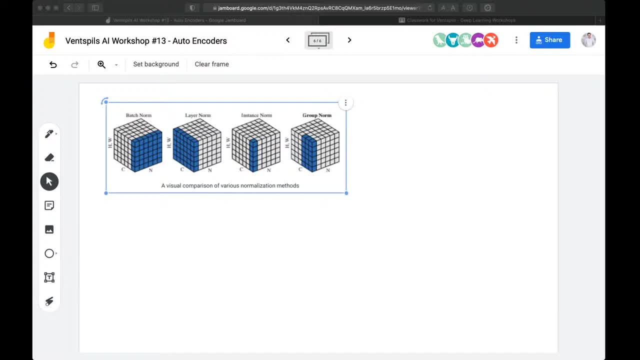 but they are necessary And maybe, like the group, norms are much better type of way to do this. So I will try to quickly, in five minutes, explain. So you have the X input. So this is in between layers. This is not X of the whole, like the very beginning. 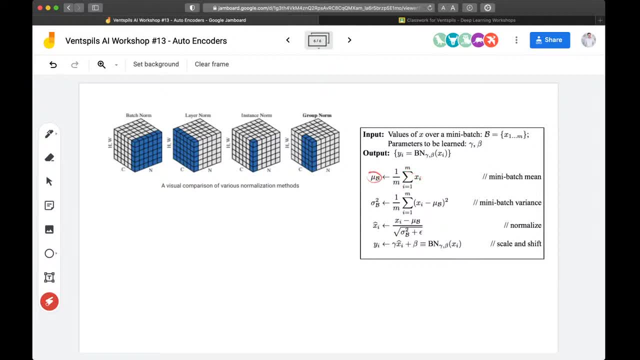 So the input, you calculate the mean here and you calculate the standard deviation, or if it's squared, then it's variance, right With regards to these means, And then we divide it, So we subtract the mean. So this is basically. 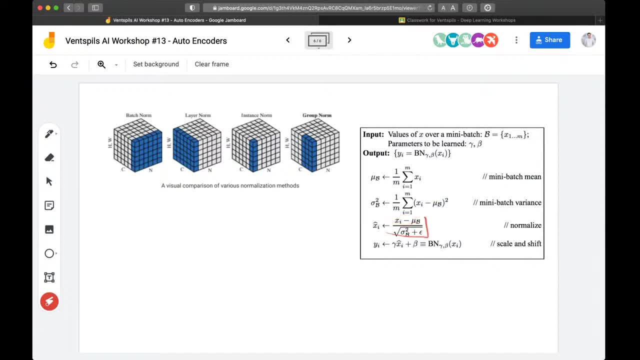 kind of similar to standardization, But the problem is that one batch doesn't represent the whole data set. That's why we need two learnable parameters, the gamma and beta. So these parameters try to be learned to represent the whole data set. 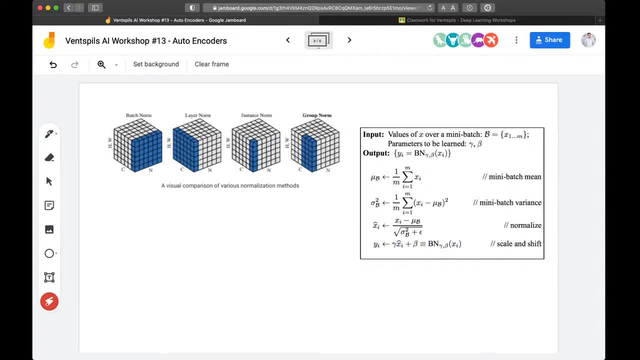 Then we arrive to another problem: that if we have two small batch sizes, then these values would jump significantly around right The variance and standard deviation, And we would not be able to learn these two values properly. So the batch sizes should be enough big enough. 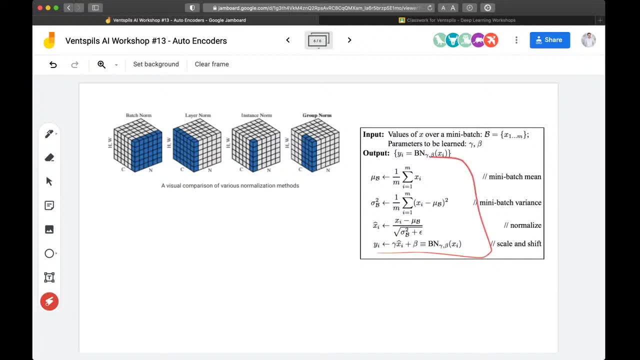 And the reason why we have all of this stuff, remember standardization. So we want to have our data to be nicely aligned. So if we again have, let's say, some kind of like X1 here, one feature X1, and there is a feature X2,. 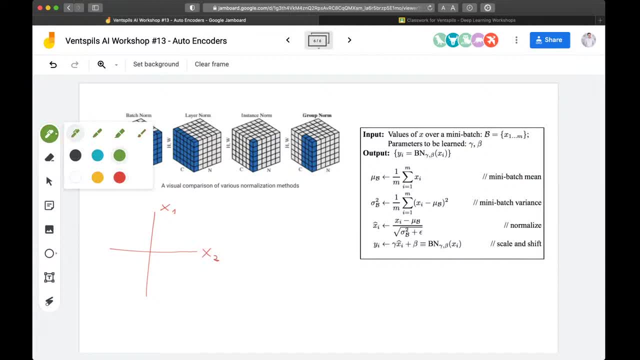 we don't want that. our features are like lying down, lying around all sorts of ways somewhere here right In one cluster. We want all of our features to be lying around the zero here. So basically the batch norm and all sorts of normalization techniques. 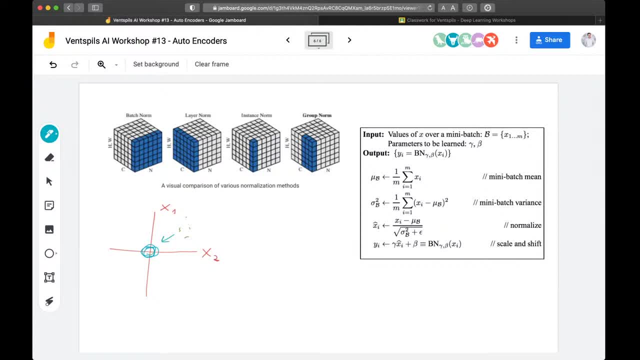 try to push our features towards the middle part so that our non-linearity function makes sense. Otherwise it doesn't make sense. So why we make it noisy? So the question about the noisy autoencoder in the chat. So the noisy autoencoder is better. 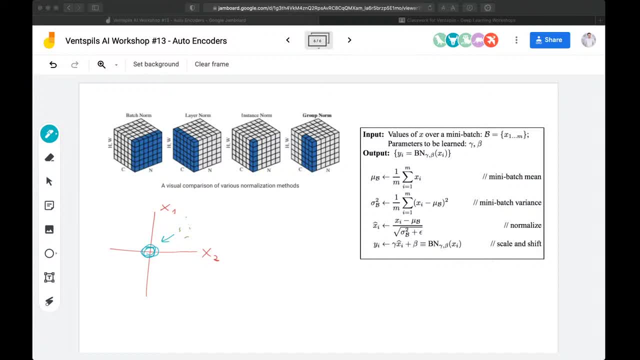 than non-noisy autoencoder. You can look up the publications and also in the reference material that I added to the 13.1, you can read that the research shows that noisy autoencoders are better. They have better embeddings. That's why there is the noisy autoencoder. 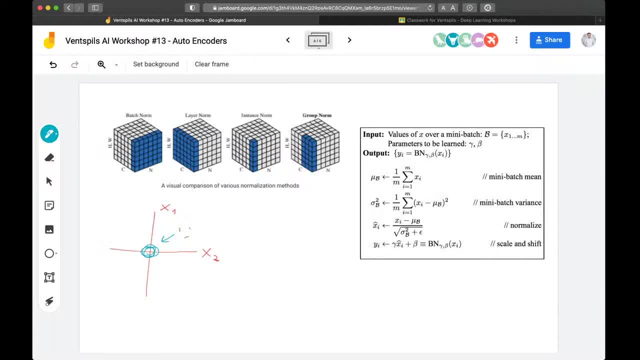 So anyway, here about the batch norm. So the batch norm is here, So you can see the N. Here are the samples. So this is samples in batch, This is N, The C is channels And the HW is the features. 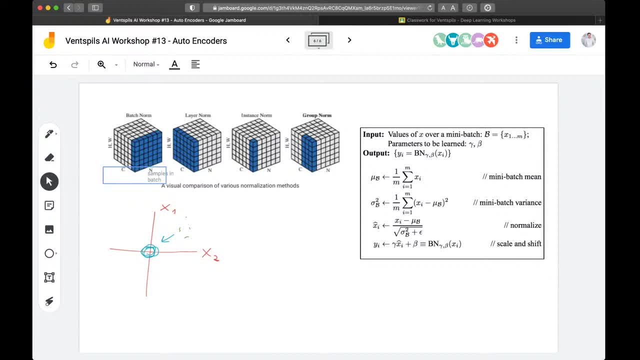 Basically the feature map sizes doesn't matter. So you see that batch norm goes over the samples of the batch, not the actually, So it's dependent on the batch size. None of the other normalization methods are dependent on the batch size. So I'll quickly try to show another example. 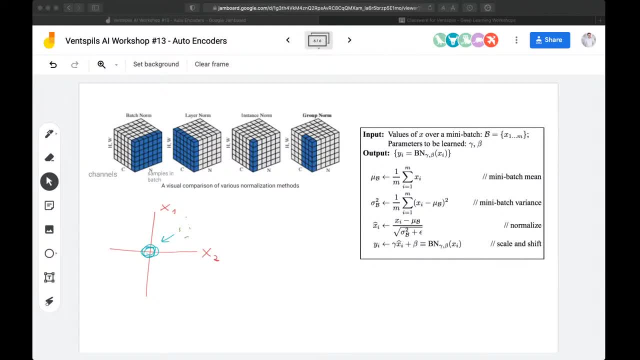 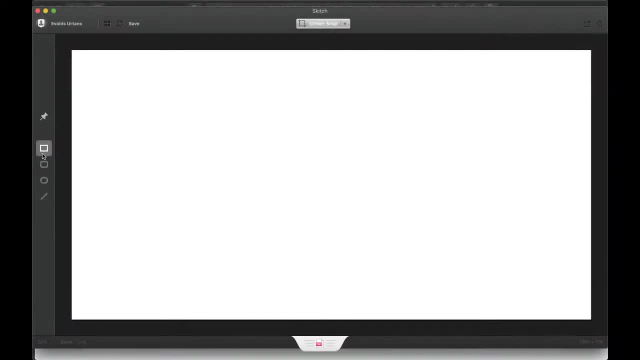 about the normalization methods that you should keep in mind. So hopefully it will work out. Let's see So if I share my whole screen and then I will post that inside the other part. So if you have the, for example, the input image of R GB green. 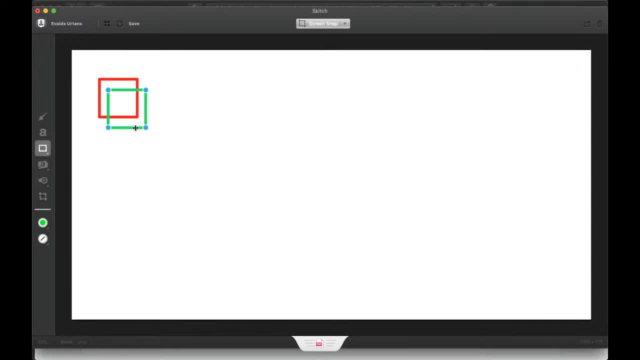 so we have three colors, right: RGB, and okay, this is G, this is B, okay, it doesn't matter. so so we have two input, three input channels and the width and height, right? so if we select our, so if we start to train this stuff and we have, let's- 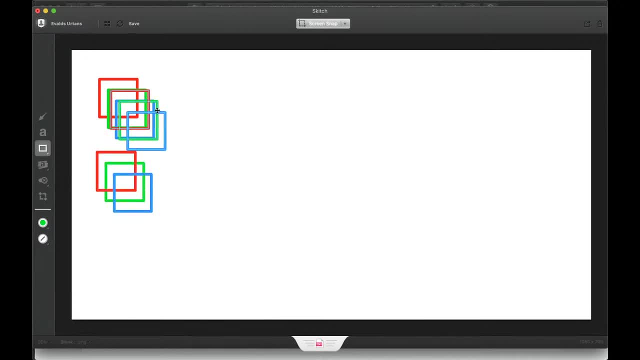 say the batch size three. so we have three sets of these, the samples. so this means that we have batch batch size three. right then, what we, what we do with the batch norm, with a batch norm, so with a batch norm. so let me also quickly copy this out so I don't miss it. so I will also show another example. 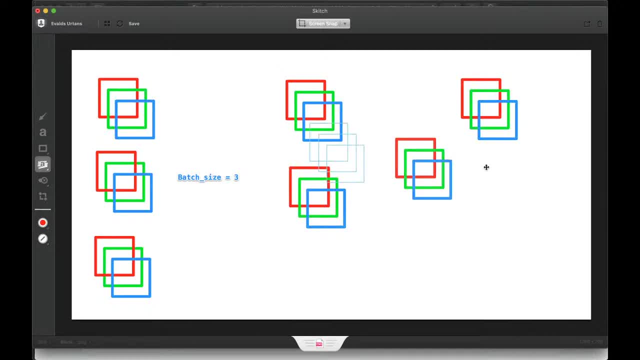 so here's. there's going to be some other examples. so the the batch norm we will be would calculate the mean and standard deviation for every channel, across every channel, for for every channel dimension. so there would be one mean value, there would be second mean value and then it will be the three mean. third mean value. 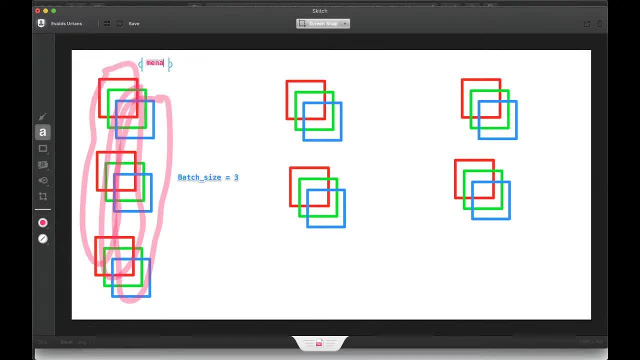 right. so there's going to be the mean mean one, two, mean three, and they are batch size dependent. so that is really bad. batch site dependence e is not what we want. so then they actually came up with the idea to have the batch norm instead of doing the batch normalization. 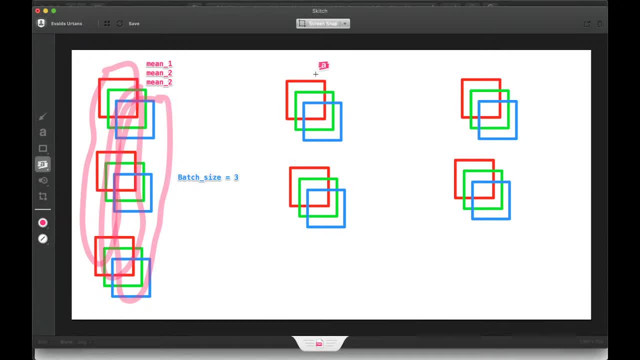 to do the layer normalization. so the the layer normalization would then calculate the mean for every single item in the batch. so they would be. so this is a layer norm, so this would cover all of these items, basically all of the all of the maps like in this direction. so, and it's not 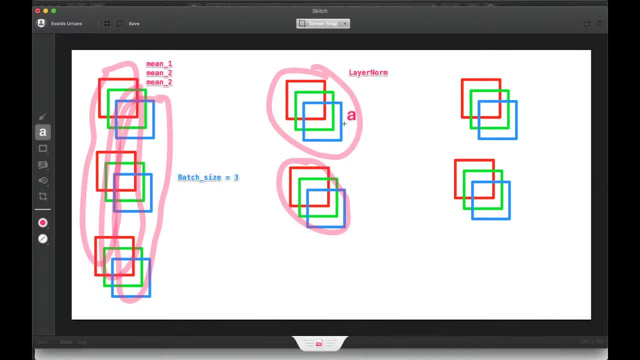 batch size dependent, so for every sample we would have just have one large mean value. Then there is also another way how to do this, using the the instance normalization, and that is by even reducing all of this problem even more. so the instance normalization would would calculate the mean value for. 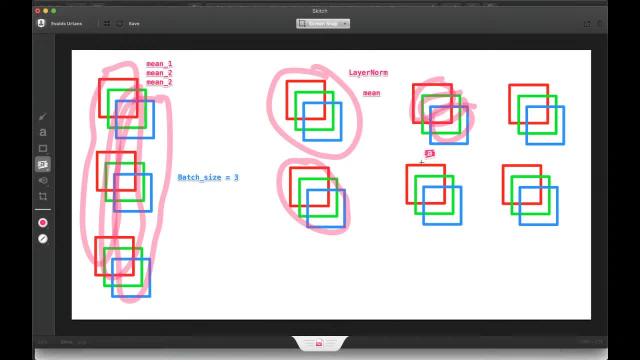 each of these maps separately, like that, but remember that all of these, these methods also look the same. So this is how you learn the, the means for whole data set. so I mean like it's not something that you would just do as a simple operation, but it will try to. 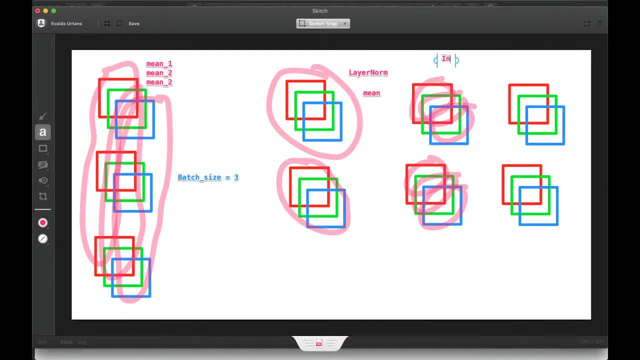 estimate what is the mean of each of those maps, for every all of the data set samples. so instance normalization: there you'd have the mean for this one, for this one, for this one, and it's- again, this is not batch size dependent. that is good. so all of these, these other methods are so far good because they are. 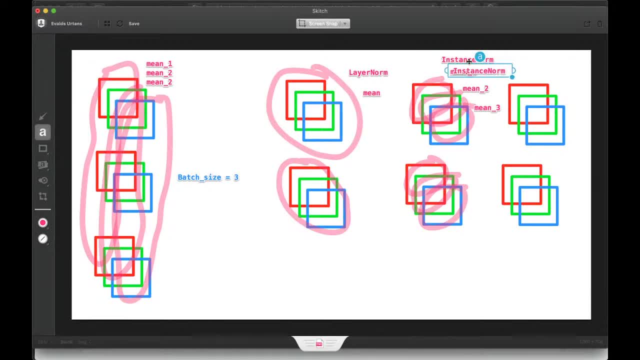 not batch size dependent. and then the third one is group norm. that you need to use actually is something in between the layer norm and the instance norm, where you select only- let's say that- some features, for example, let's say the some, you would have some kind of red object on the scene of. 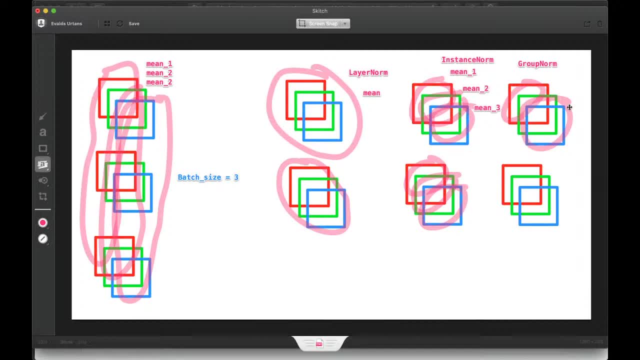 of blue and green valley. you know like there's a, there's a lake and there's like mountain right and then there is a red car right. so you would have that these two. these two are together and this is separate. so the fun thing is that the 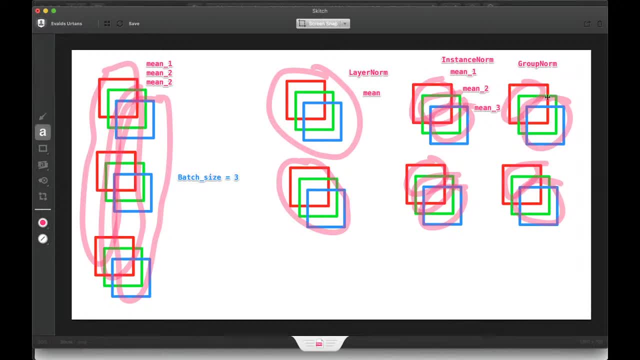 neural network models will learn how to split those. but if you just say that we would want to have num two groups, it would automatically learn to put together those features in one group and other group. so that's why you should use always group norm and you should do the 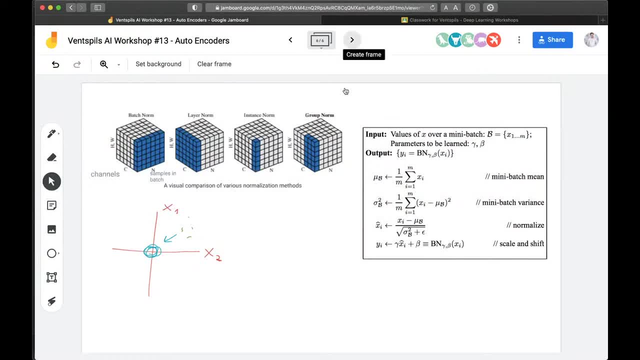 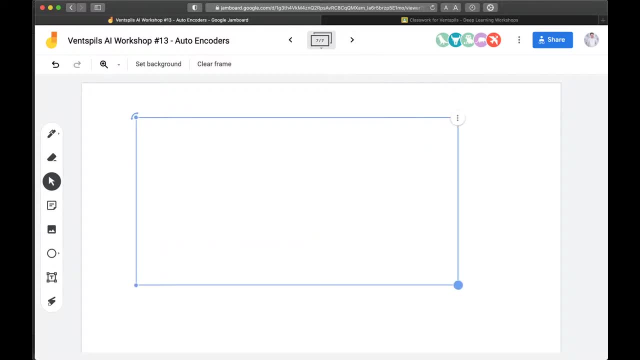 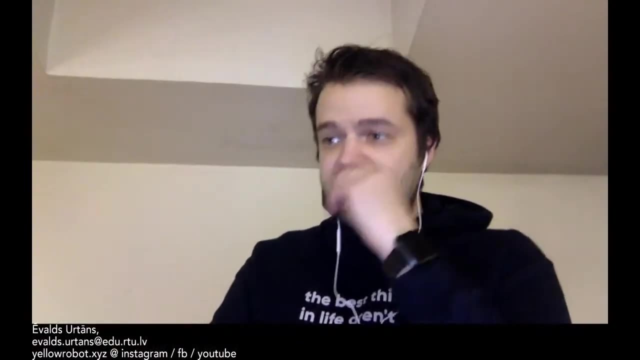 experiments and find the best value for for the number of groups. so this is again new hyper parameter, but this is a good thing because it's not batch size dependent. so yeah, so this is this. so if you have questions with regards to these normalization techniques, then please just like write in the whatsapp group or 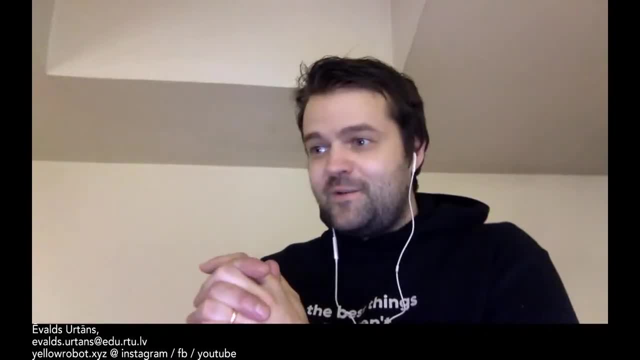 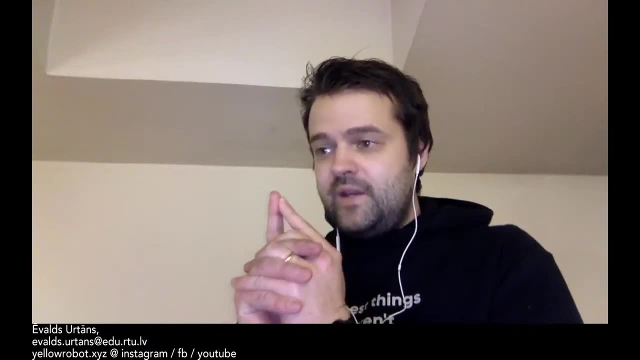 whatever, and I can help you out with that, but now I need to run, so I will put the homework in the Google classroom, so it will be probably fun and yeah, so. so next time we will keep working on the auto encoders and then, time after that, we will start working on 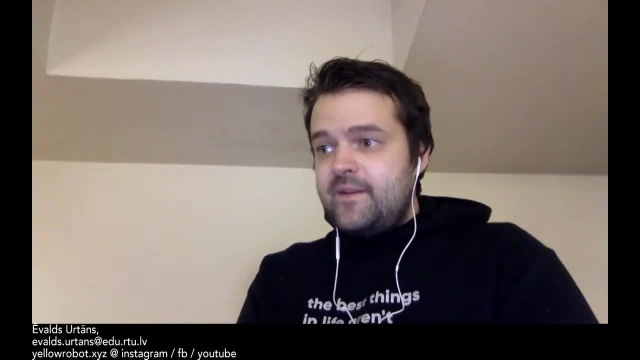 the units. that's it for the day. I hope it was fun and yeah, let me know. 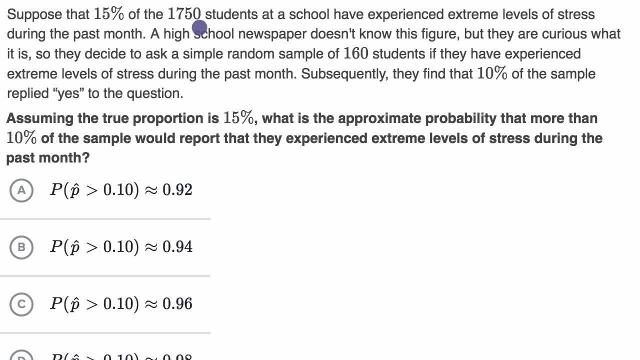 We're told, suppose that 15% of the 1,750 students at a school have experienced extreme levels of stress during the past month. A high school newspaper doesn't know this figure, but they are curious what it is, so they decide to ask a simple, random sample of 160 students. 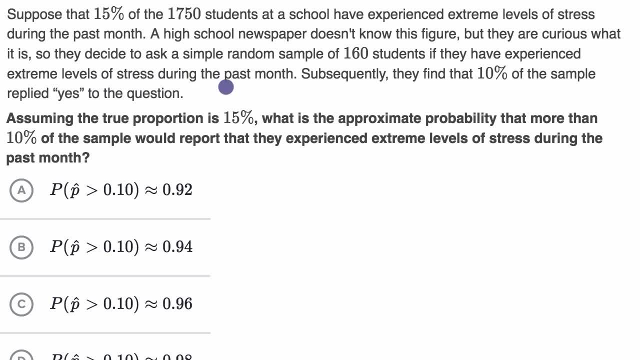 if they have experienced extreme levels of stress during the past month. Subsequently, they find that 10% of the sample replied yes to the question, Assuming the true proportion is 15%, which they tell us up here they say 15% of the population. 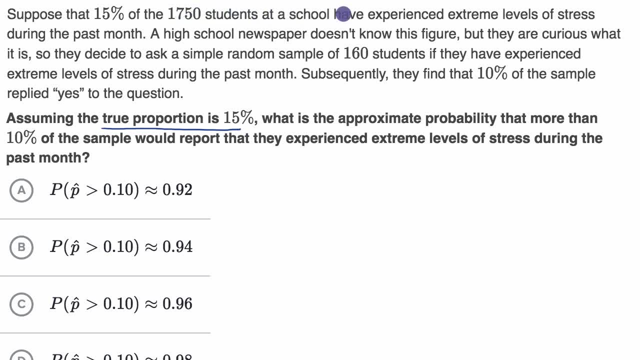 of the 1,750 students actually have experienced extreme levels of stress during the past month. So that is the true proportion. So let me just write that The true proportion for our population is 0.15.. What is the approximate probability? that more than 10% of the sample.